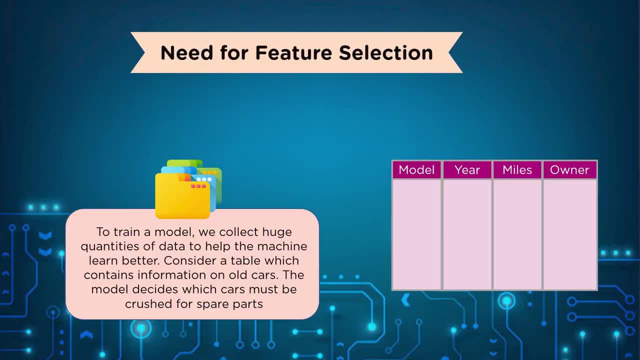 talk about huge quantities of data. they save everything from people's favorite cat pictures to- and you can imagine there's so much data out there. Even in a company, they'll save all these little pieces of information about what's in it for you. So the need for feature selection. 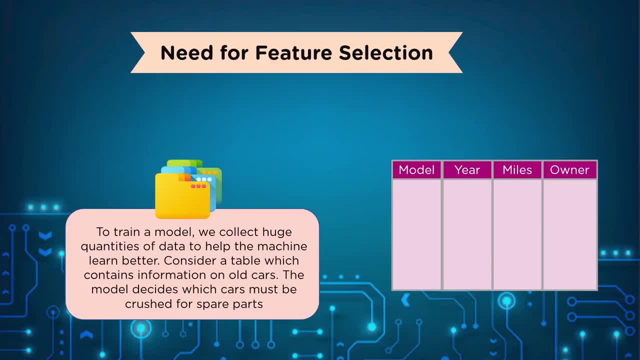 So when you talk about what's in it for an industrial opportunity, like your door lock, you need some important data loss area So you don't really need to have to worry about people and companies and corporations. You need some way to sort through because if you try to, 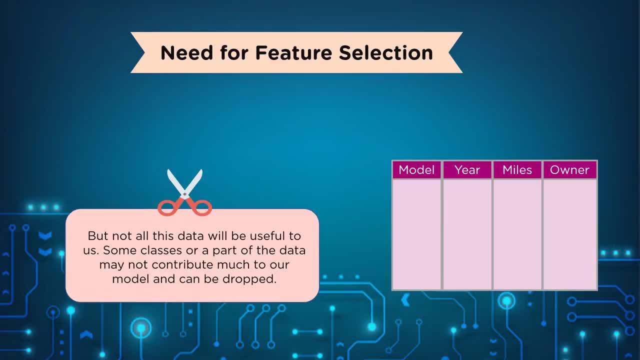 run your models on all of it. you'll end up with these very clunky models and they might have issues which we'll talk about later, But in this case we're talking about cars and crushing. But not all this data will be useful to us. Some classes or part of the data may not contribute. 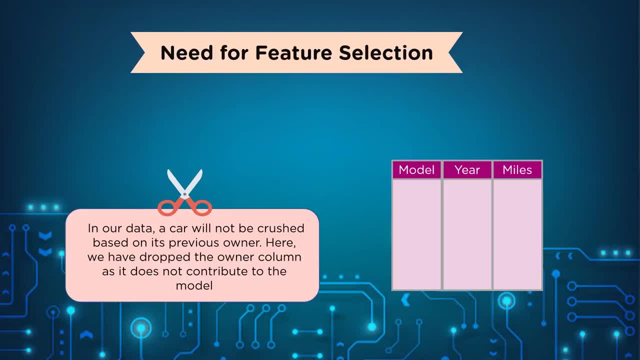 much to our model and can be dropped And you can see right here we have who was the owner of the car. So that's kind of a clear cut. You can see that. Why would I care who owned the car before Once? 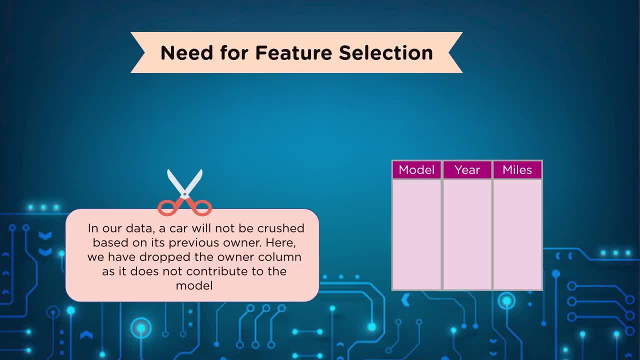 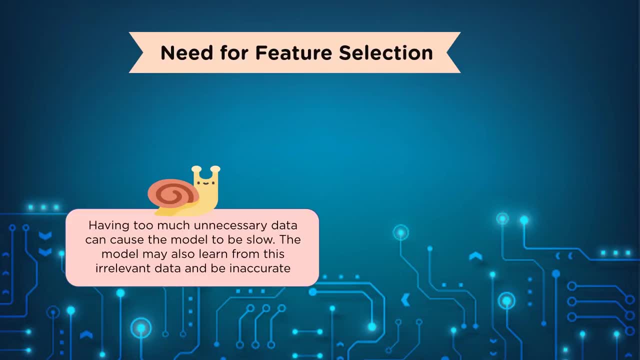 it's in the junkyard and we're crushing the cars. we're not going to really care about that. So here we have dropped the owner column, as it does not contribute to the model. Having too much unnecessary data can cause the model to be slow. The model may also learn from this irrelevant data. 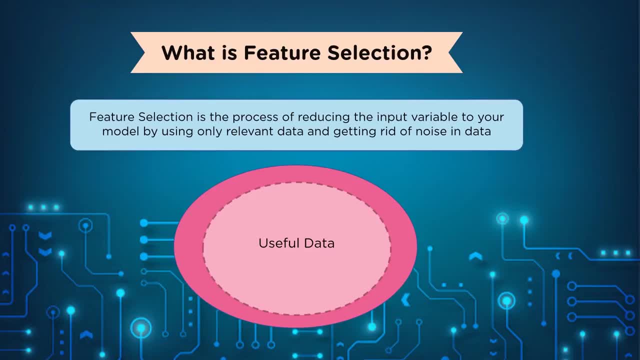 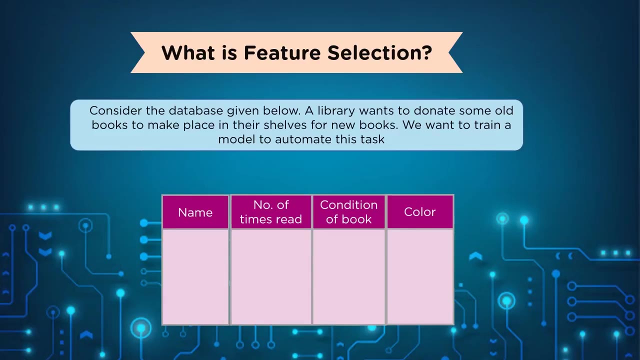 and be inaccurate. So feature selection is a process of reducing the input variable to your model by using only relevant data and getting rid of the noise in the data. Consider the database given below. A library wants to donate some old books to make place in their shelves for new. 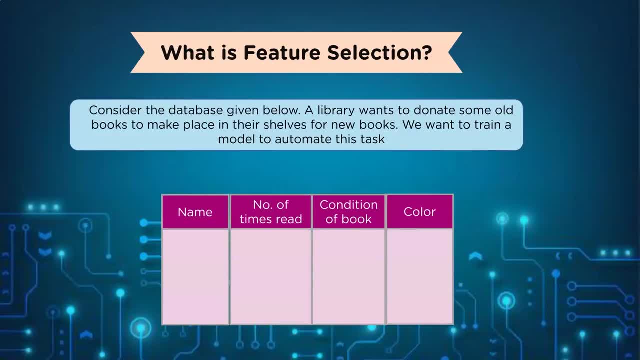 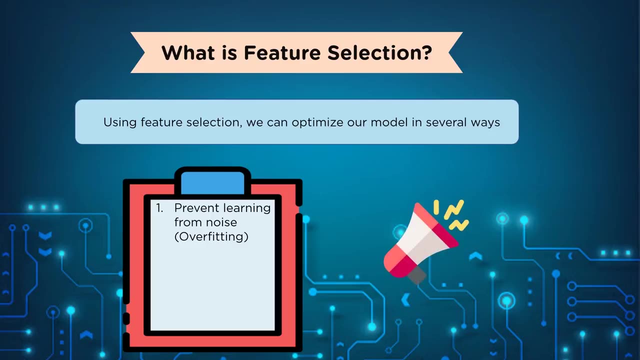 books. We want to train a model to automate this task. In this case, the color of the book does not matter, and keeping it can cause a model to learn to donate books based on color. We can remove this as a feature Using feature selection. we can optimize our model in several ways, And so 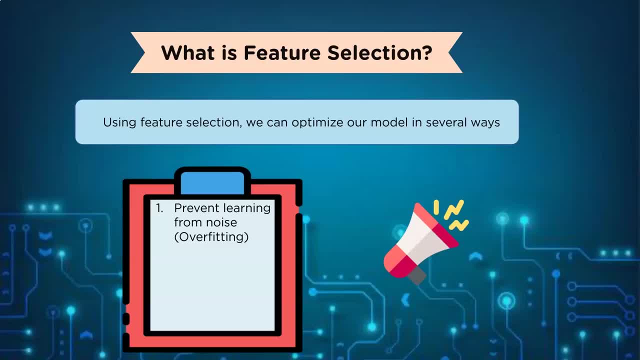 the number one is to prevent learning from noise and overfitting. That's actually the huge one, because we don't want it to give us the wrong prediction, And that means also improved accuracy. So, instead of giving us a wrong prediction, we also want it to be as close to the right. 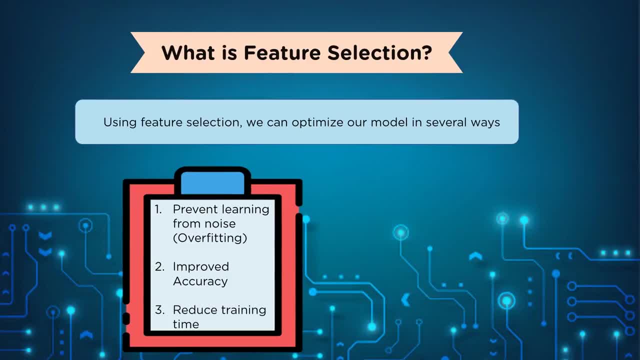 answer: as we can get, And we want to reduce the training time. It's an exponential growth in some of these models, So each feature you add is going to be a different one. So we want to reduce the training time. We want to increase the number of features that we add, So that's a much better. 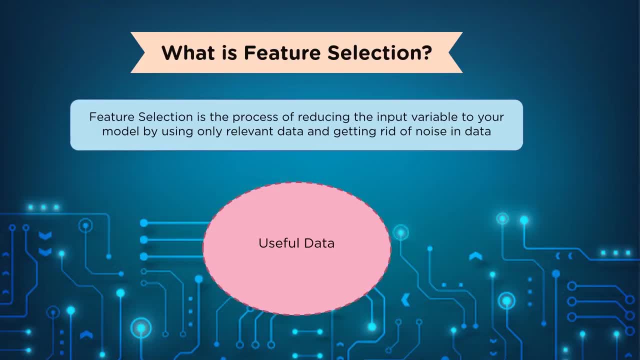 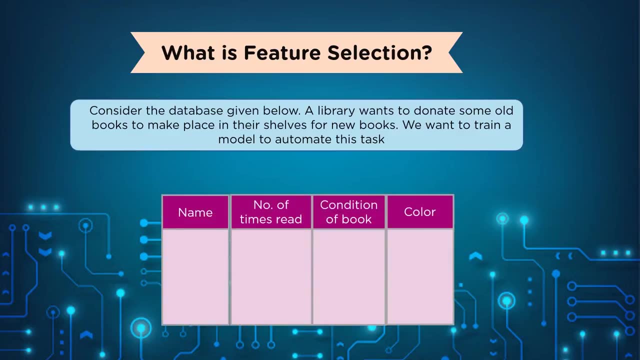 to your model by using only relevant data and getting rid of the noise in the data. consider the database given below. a library wants to donate some old books to make place in their shells for new books. we want to train a model to automate this task. in this case, the color of the book does not matter in 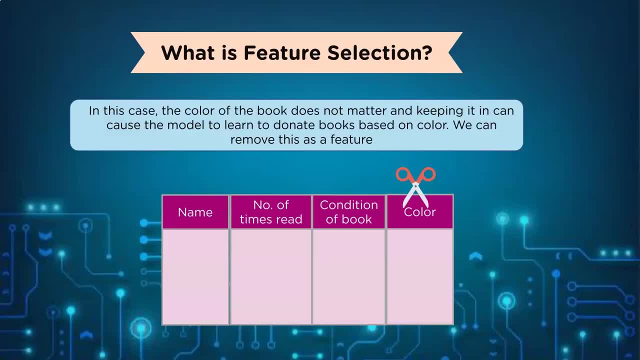 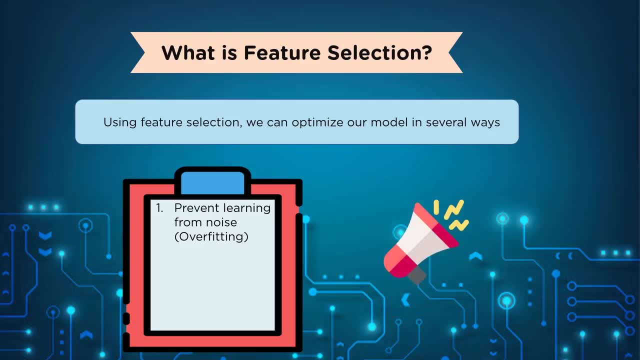 keeping it can cause a model to learn to donate books based on color. we can remove the model from the database and then use the model to automate the model. we can optimize our model in several ways, and so the number one is to prevent learning from noise and overfitting. that's actually the huge one. 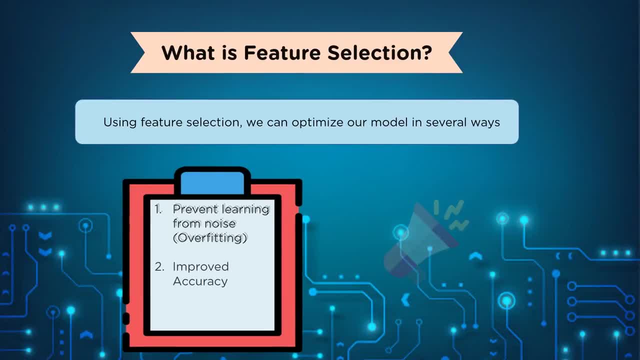 because we we don't want it to give us the wrong prediction, and that means also improved accuracy. so instead of giving us a wrong prediction, we also want it to be as close to the right answer as we can get, and we want to reduce the training time. it's an exponential growth in some of these models, so the each 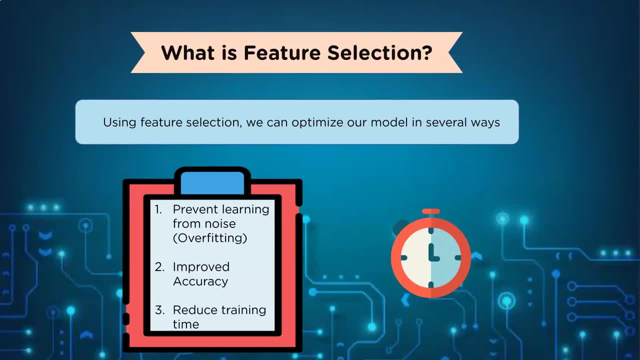 feature you add in includes the number of books that you can donate to the library for a particular reason, whether it's just for you or the library has access to the library. we want to use the information that you can use to integrate your method and the information that you can use to 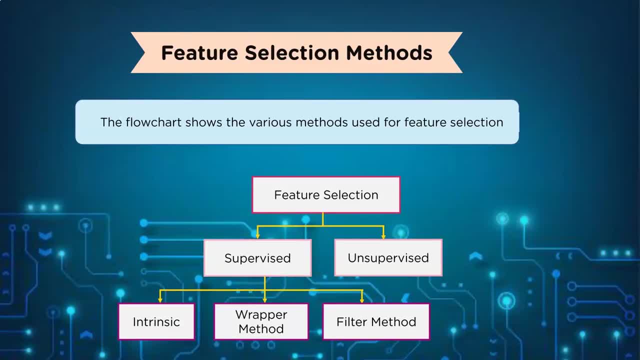 integrate your method and the information you can use to integrate your method can be used to convert a lecture into a real text and then hopefully use them in the future as well. so the number of books you add in increases that much. more training time: we talked about feature selection methods. 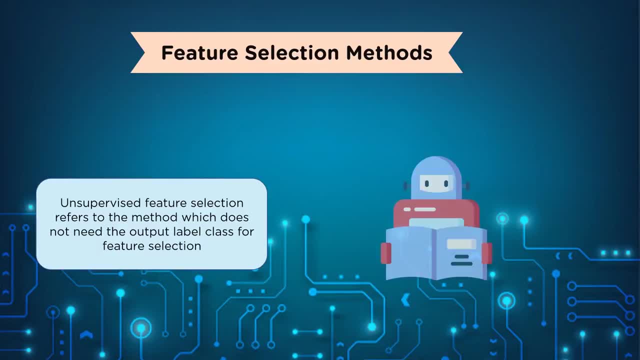 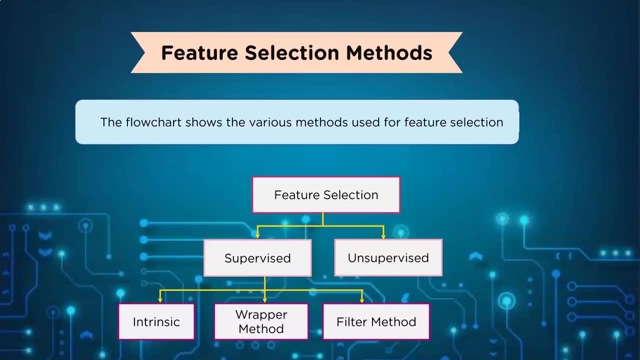 we put together a nice little flowchart that shows the various methods used for feature selection and you have your basic feature selection and then there is class for feature selection and that was you can see here under super unsupervised. we don't have- that's really a growing market right now- unsupervised learning, and so feature selection. 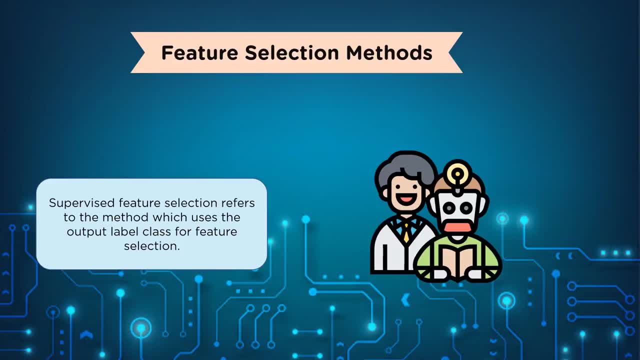 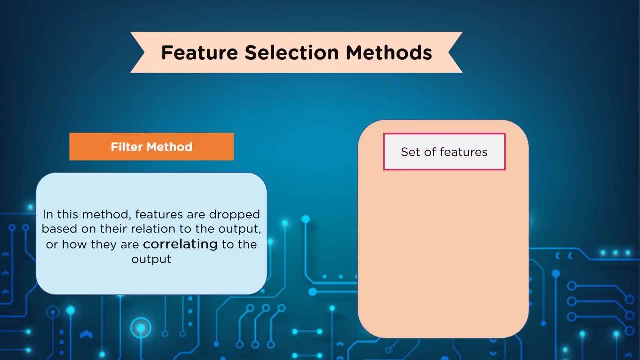 is the same thing. supervised feature selection refers to the method which uses the output label class for the feature selection and, if you remember, we looked at three different. we have intrinsic wrapper and filter method, so we're gonna start with the filter method on this now. remember we 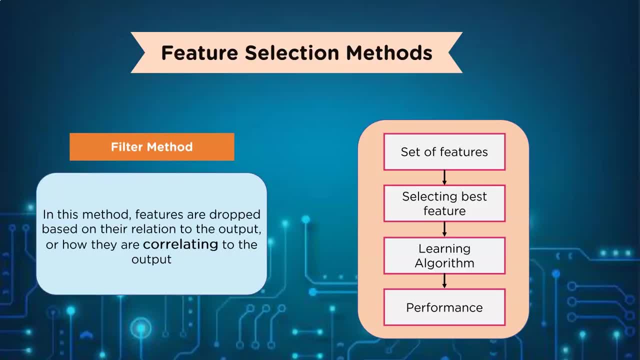 know what the output is, so we're gonna be looking at that output to see how well it's doing versus the features. in this method, features are dropped based on their relation to the output or how they are correlating to the output. you can see here we have a set of features, selecting best feature. 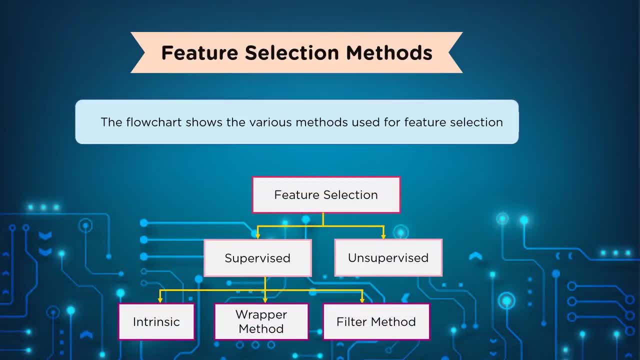 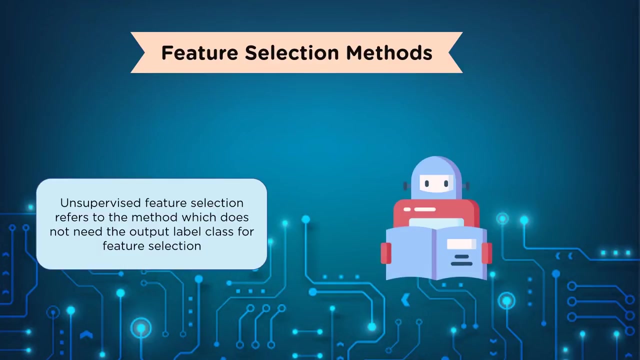 result: We talk about feature selection methods. We put together a nice little flow chart that shows the various methods used for feature selection And you have your basic feature selection. and then there is supervised and unsupervised. Under supervised there's intrinsic wrapper method, filter method. So we talk about unsupervised. feature selection refers to the 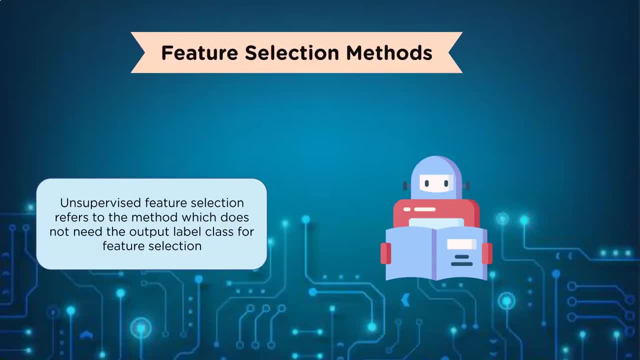 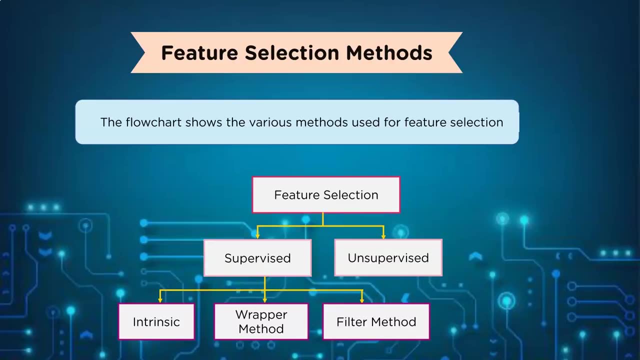 method which does not need the output label. And then we talk about the method that uses the class for feature selection, And that was you can see here under unsupervised. we don't have- that's really a growing market right now- unsupervised learning And so feature selection. 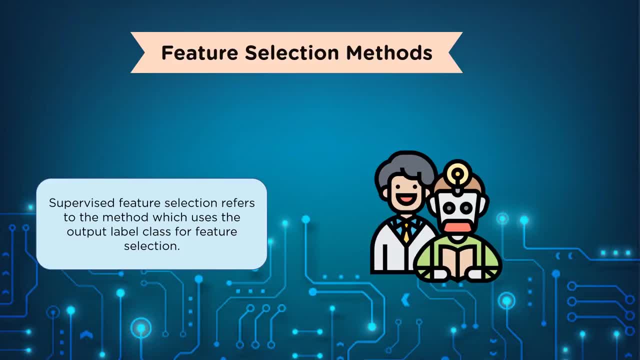 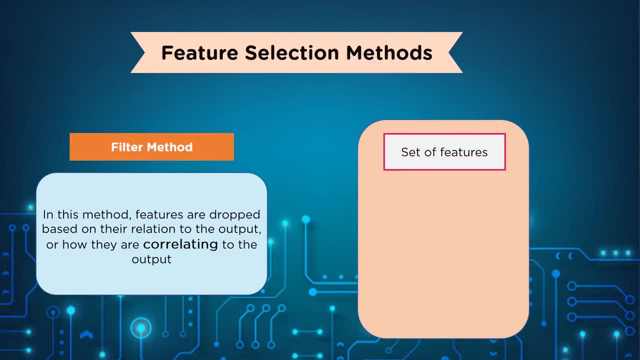 is the same thing. Supervised feature selection refers to the method which uses the output label class for the feature selection And, if you remember, we looked at three different. we have intrinsic wrapper and filter method, So we're going to start with the filter method on this. 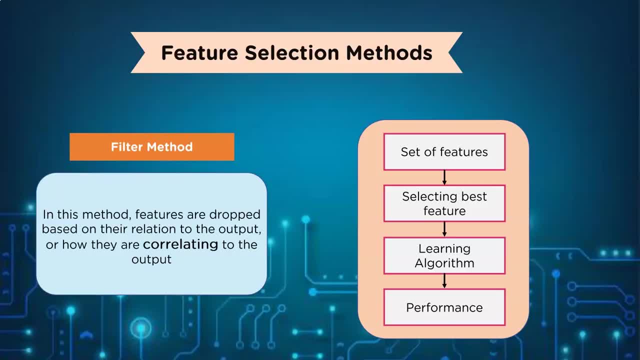 Now remember, we know what the output is, So we're going to be looking at that output to see how well it's doing versus the features. In this method, features are dropped based on their relation to the output or how they are correlating to the output, And you can see here we have a set. 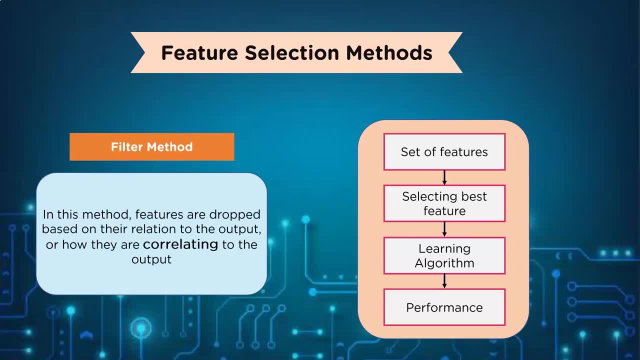 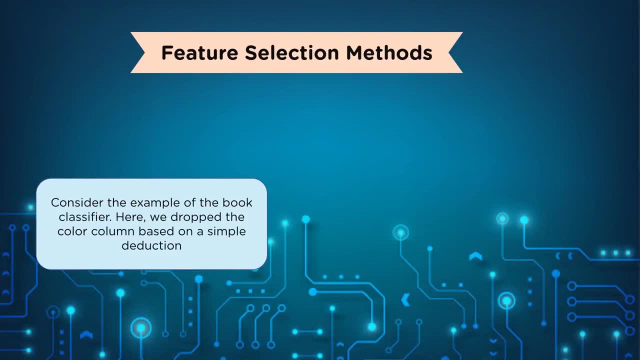 of features, selecting best feature learning algorithm, and then performance, And so we want to find out which feature correlates to the performance on the output. Consider the example of book classifier. Here we drop the color column based on simple deduction, And that kind of sums it up in a nutshell is we want to filter out things. 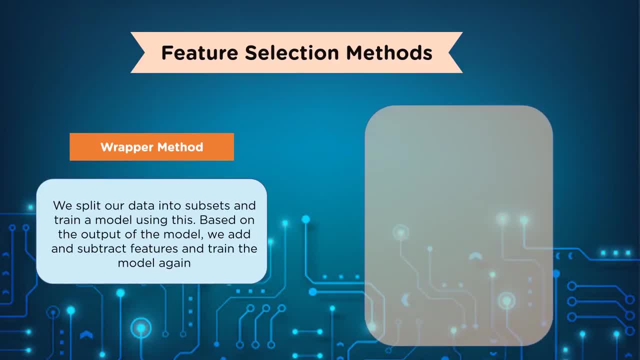 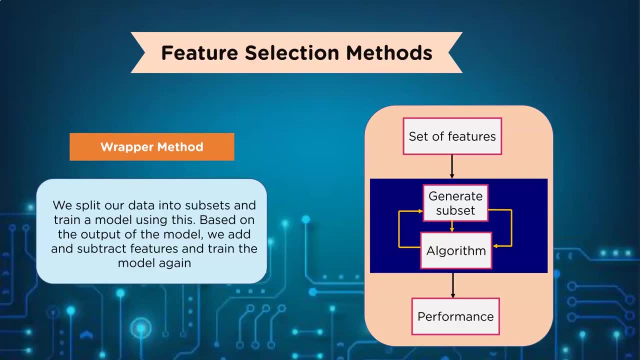 that clearly do not go with what we're looking for. We look at the wrapper method. In the wrapper method, we split our data into subsets and train a model. using this, Based on the output of the model, we add and subtract features and train the model again And you can see here in the wrapper: 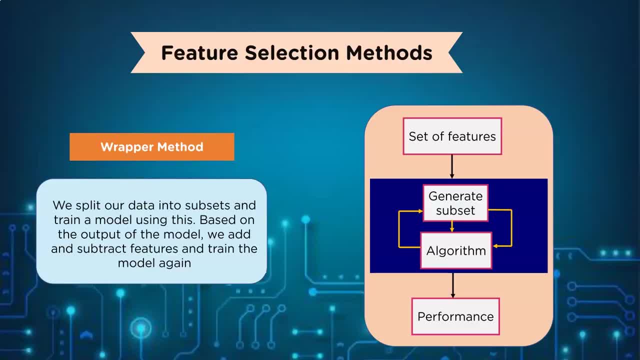 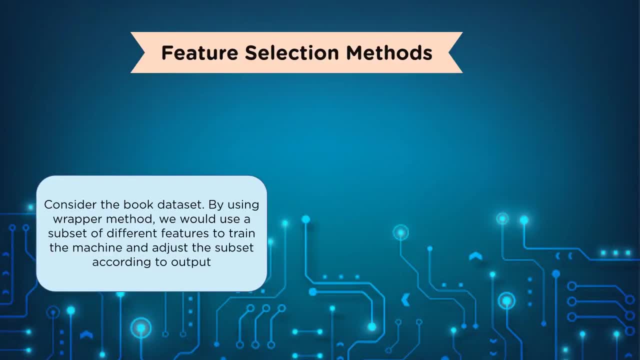 method. we have a set of features, we generate a subset, we run it through the algorithm and we see how each one of those features are correlated to the output, And so we want to filter out which subset of features performs. Consider the book data set By using the wrapper method we would. 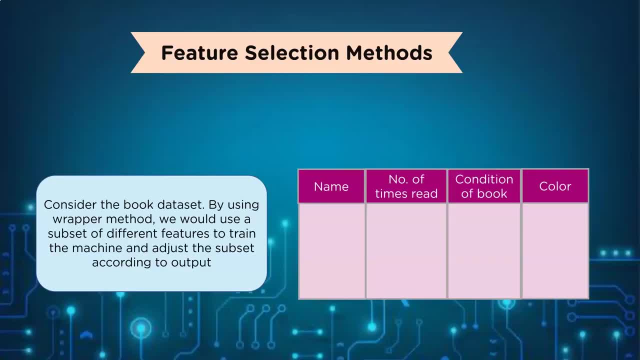 use a subset of different features to train the machine and adjust the subset according to the output. And so you can see here, let's say we take name and number of times read and we run just those and we look at the output. And if we looked at them with all four inputs, and look at the output, 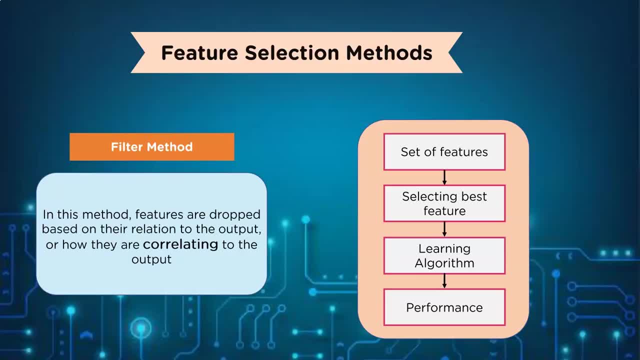 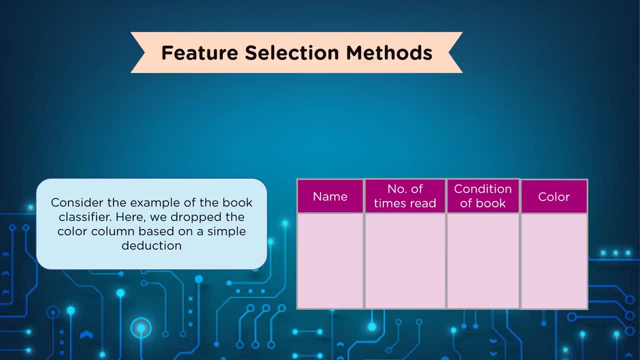 learning algorithm and then performance, and so we want to find out which feature correlates to the performance on the output. consider the example of book classifier. here we drop the color column based on simple deduction, and that kind of sums it up in a nutshell is: we want to filter out things that clearly do not go with what we're looking. 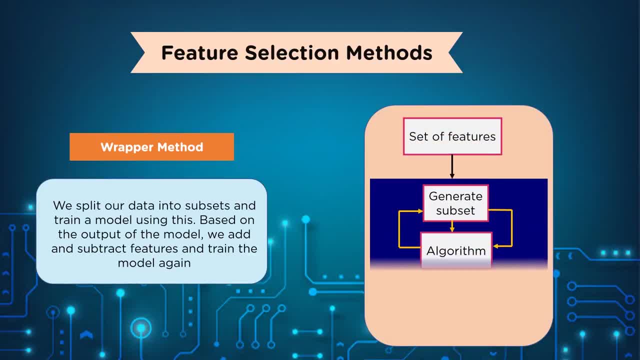 for we look at the wrapper method. in the wrapper method we split our data into subsets and train a model using this. based on the output of the model, we add and subtract features and train the model again. and you can see here in the wrapper method we have a set of features, we generate a subset. 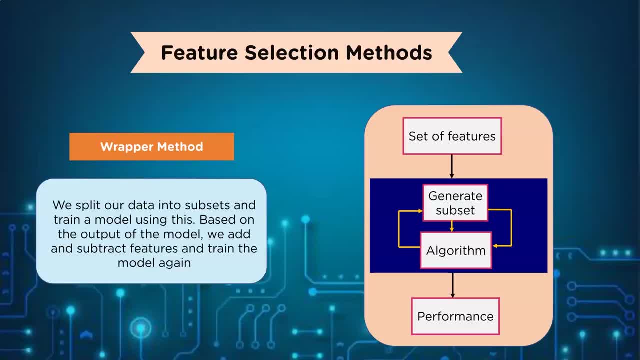 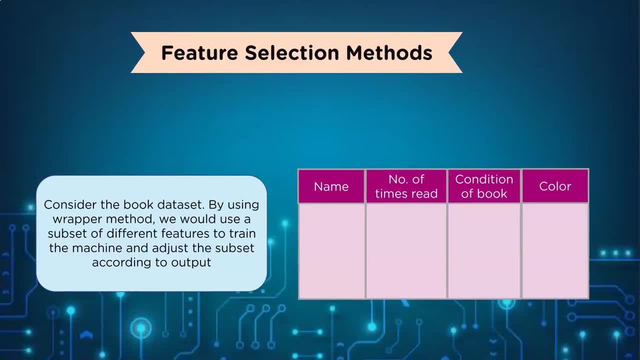 we run it through the algorithm and we see how each one of those subset of features performs forms. Consider the book data set. By using the wrapper method, we would use a subset of different features to train the machine and adjust the subset according to the output. 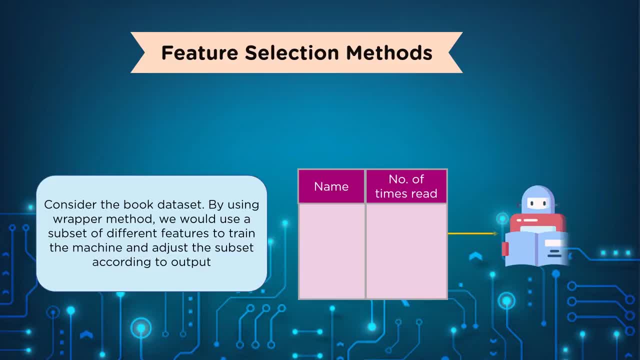 And so you can see here, let's say, we take name and number of times read and we run just those and we look at the output. And if we looked at them with all four inputs and look at the output, we'd see quite a different variation in there and we might say you: 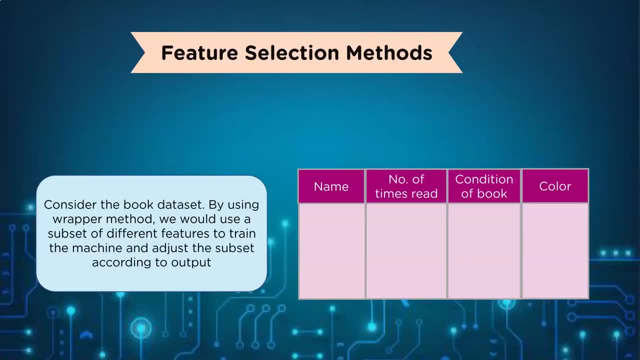 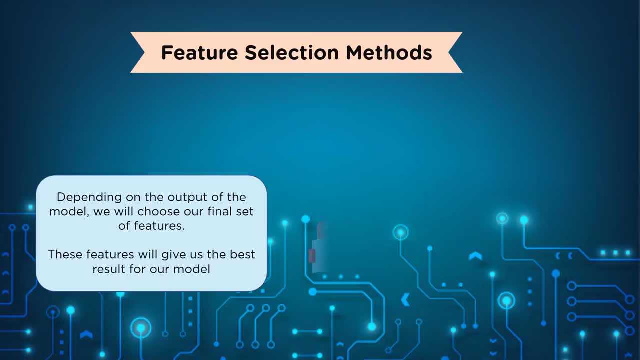 know what condition of the book and color really doesn't affect what we're looking for And you can see here we've run it on condition of the book and color. Depending on the output of the model, we will choose our final set of features. These features will give us the 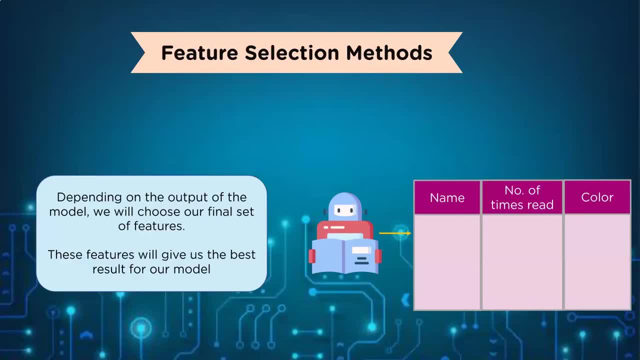 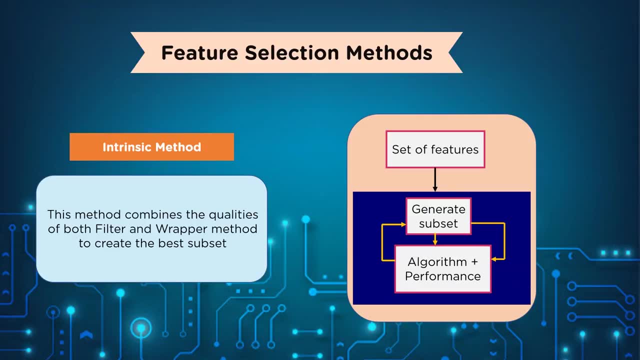 best result for our model And it might come up that the name number of times read is probably pretty important. The intrinsic method: this method combines the qualities of both filter and wrapper method to create the best subset. The model will train and check the 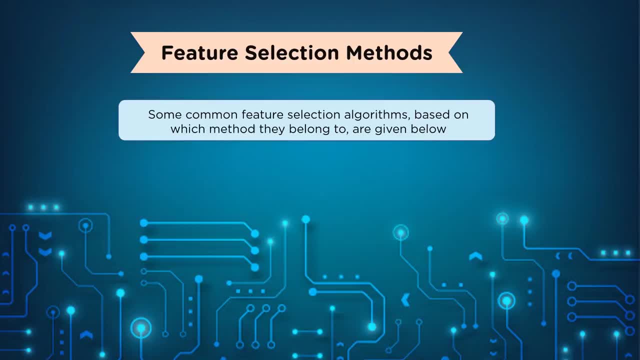 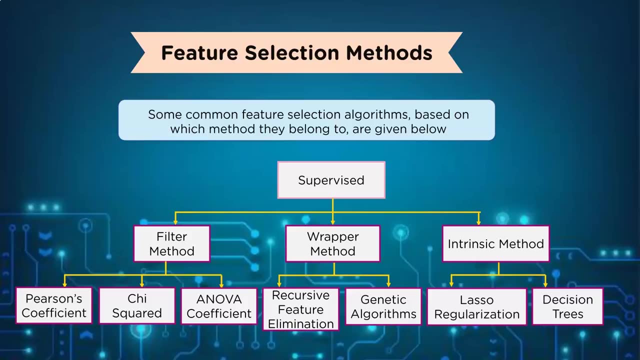 accuracy of different subsets and select the best among them. We kind of looked at a little overview. Here's some of the stuff. Some of the common feature selection algorithms, based on which method they belong to, are given below And you'll see it's primarily under supervised. 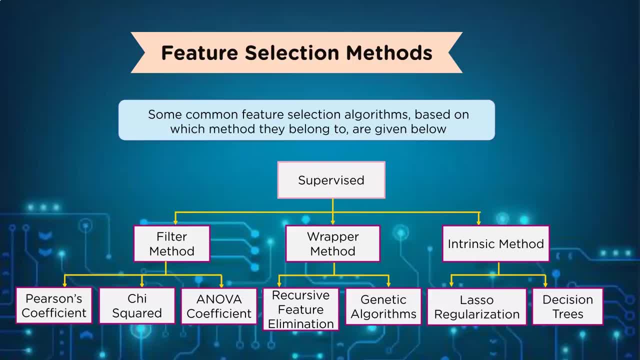 There's not, like I said, a lot of unsupervised methods, and the ones that are usually use these methods and finds a way to create a supervised connection between the data. And when we talk about supervised methods, we have our filter method, which we talked. 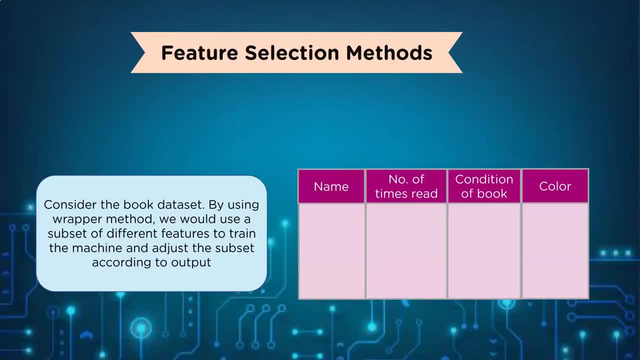 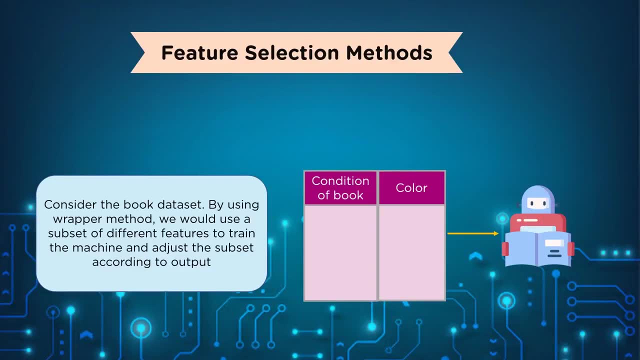 we'd see quite a different variation in there And we might say, you know what condition of the book and color really doesn't affect what we're looking for. And so we're going to look at the output and see what we're looking for And you can see here we've read it on condition of the book and color. 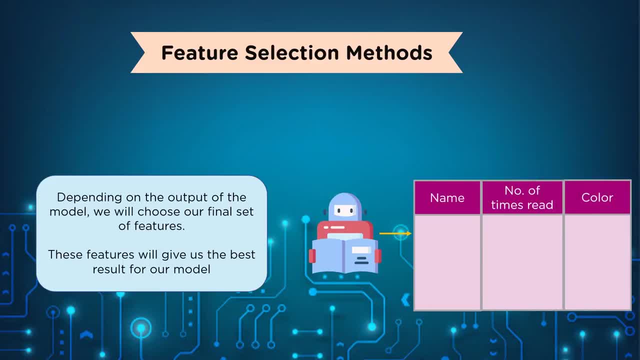 Depending on the output of the model, we will choose our final set of features. These features will give us the best result for our model, And it might come up that the name number of times read is probably pretty important. The intrinsic method: this method combines the qualities of both filter. 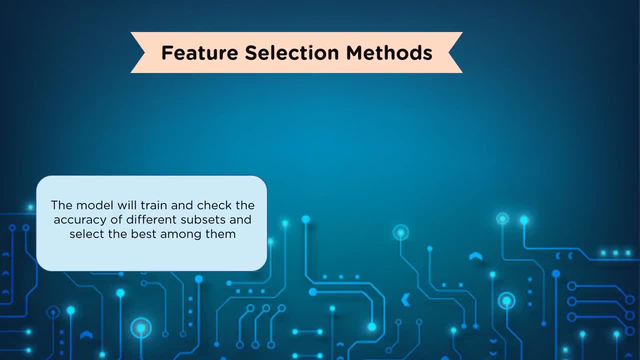 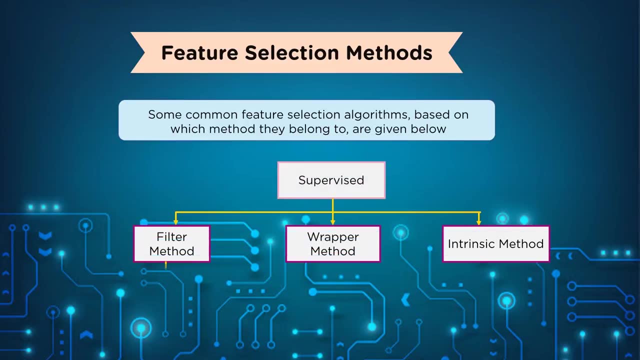 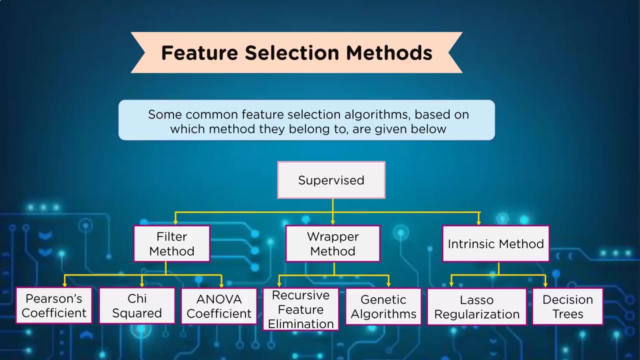 and wrapper method to create the best subset. The model will train and check the accuracy of different subsets and select the best among them. We kind of looked at a little overview of some of the stuff. Some of the common feature selection algorithms based on which method they belong to, are given below And you'll see it's primarily under supervised. 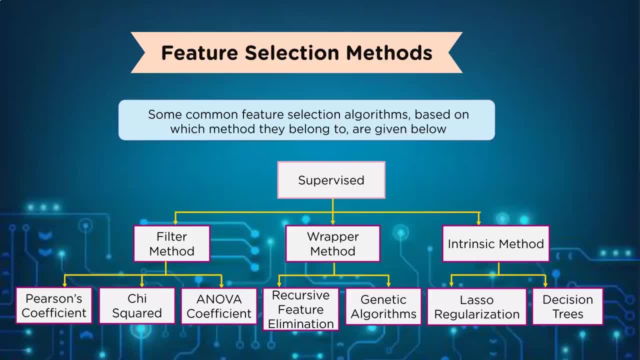 There's not, like I said, a lot of unsupervised methods, And the ones that are usually use these methods and finds a way to create a supervised connection between the data. And we talk about supervised methods. we have our filter method, which we talked about, And it uses like the Pearson's coefficient. 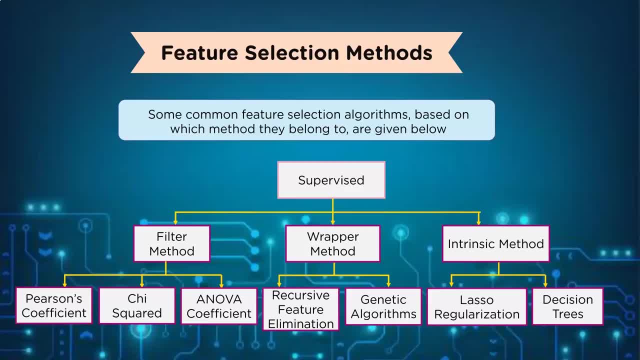 chi squared ANOVA coefficient. Those are all under the filter method And in the wrapper method, recursive feature elimination. So remember, we're choosing a subset and we want to go through there and look at each one. So you're just doing a lot of loops or recursive calculations to see which one works best and which ones don't have an impact on the output. 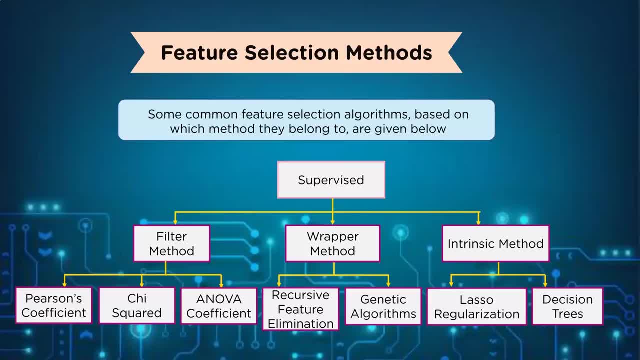 And there's a lot of genetic algorithms to go with this too, on the wrapper method and how they evaluate it, And with the intrinsic method. there's the two main ones we're looking at. One is the lasso regularization. The lasso algorithms are basically your standard regression model. 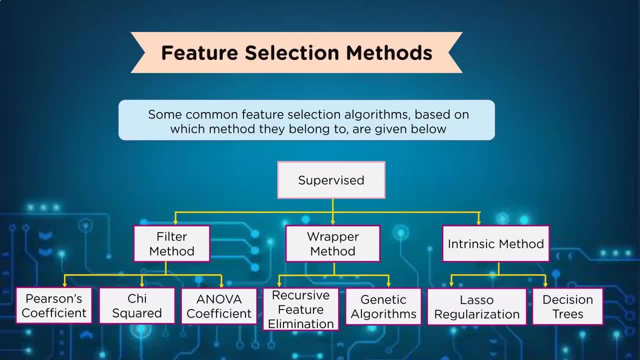 So it's finding out how these different methods fit together and which ones have the best add together to have the least amount of error. The other one used in the intrinsic method is the decision tree. It says, hey, if this one produces this result. 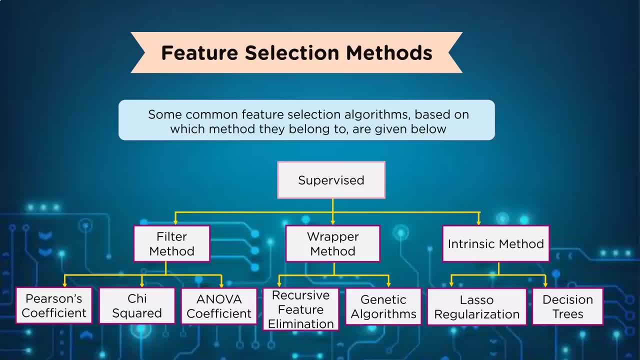 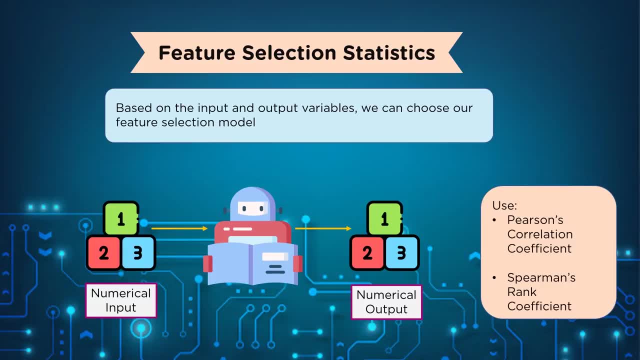 this one produces this result: yes, no. which way do we go? Based on the input and the output variables, we can choose our feature selection model. You have your numeric input coming in. you have your numeric output If you use the. 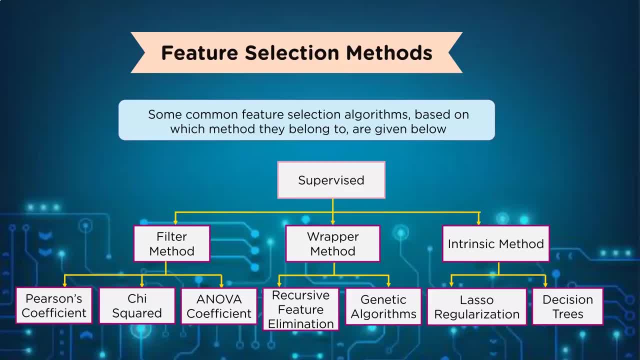 about and it uses, like the Pearson's coefficient chi-squared, A nova coefficient. Those are all under the filter method And in the wrapper method, recursive feature elimination. So remember, we're choosing a subset and we want to go. 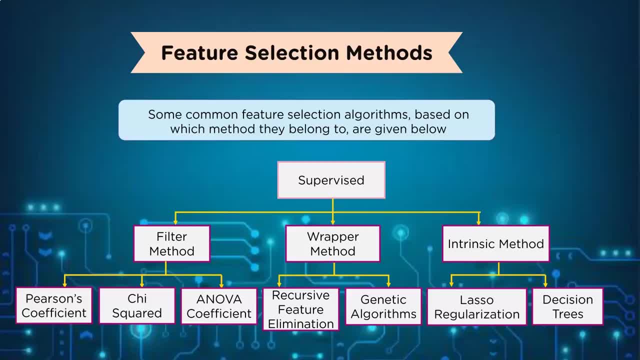 through there and look at each one. So you're just doing a lot of loops or recursive calculations to see which one works best and which ones don't have an impact on the output. And there's a lot of genetic algorithms to go with this too, on the wrapper method and how they evaluate. 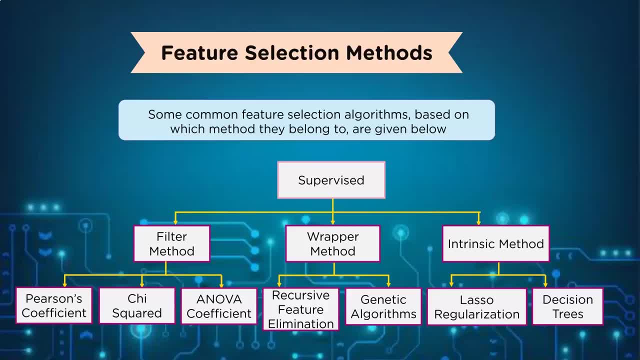 it, And with the intrinsic method there's the two main ones we're looking at is the lasso regularization. The lasso algorithms are basically your standard regression model, So it's finding out how these different methods fit together and which ones have the best add together. 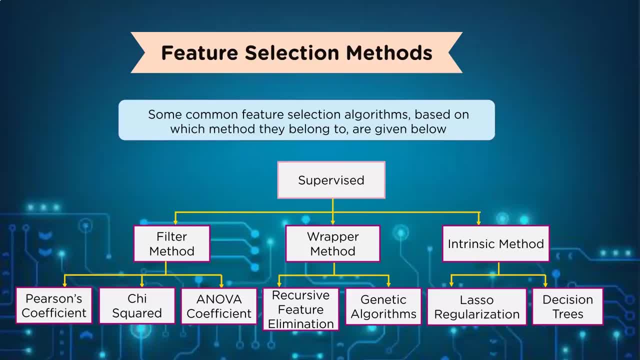 to have the least amount of error. The other one used in the intrinsic method is the decision tree. It says: hey, if this one produces this result, this one produces this result. yes, no. which way do we go? Based on the input and the output variables, we can choose our 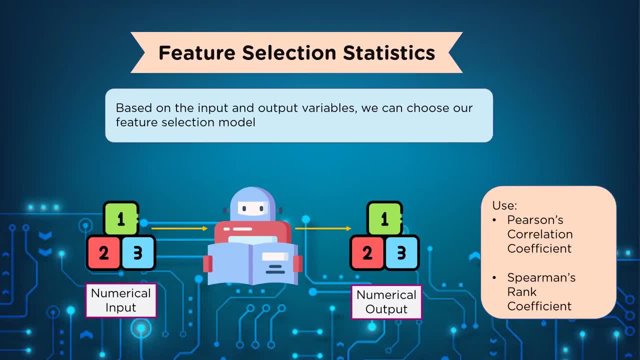 feature selection model And then we can go back and look at the output variables. So you have your numeric input coming in. you have your numeric output If you use the Pearson's correlation coefficient or Spearman's rank coefficient. you can then select what features. 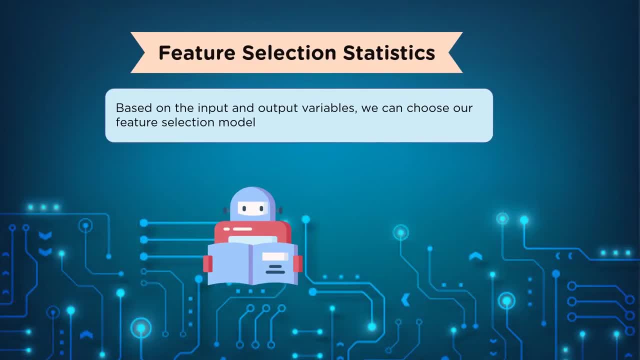 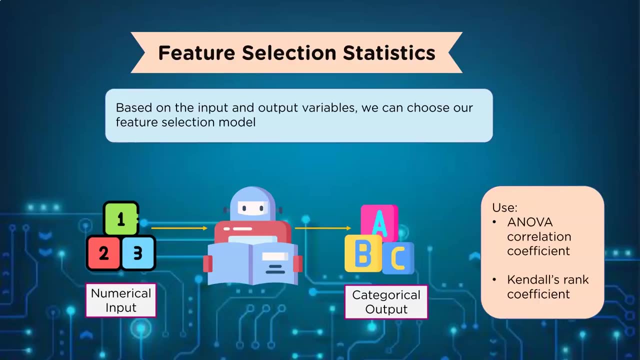 you're going to feed into that specific model And you maybe have a numerical input and a categorical input. so we're going to be looking more at a NOVA correlation coefficient or Kendall's rank coefficient And if you have a categorical input and a numerical output, 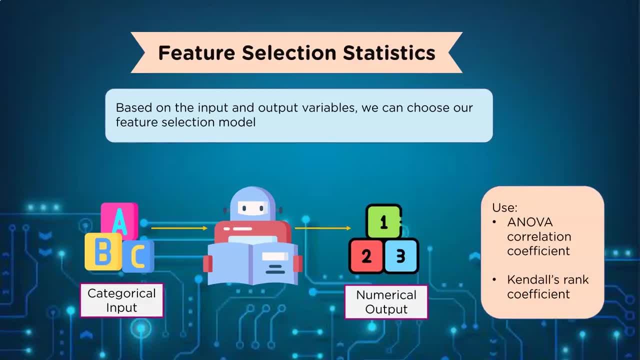 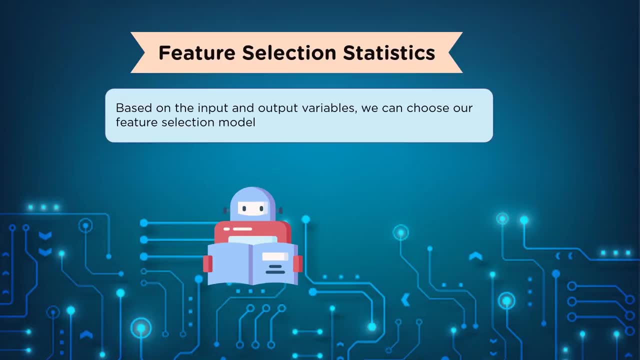 we might be looking at a NOVA correlation coefficient and Kendall's rank coefficient. So based on the input and the output variables we can choose our feature selection model And you can see we have categorical to categorical. We might be looking at the chi-squared test. 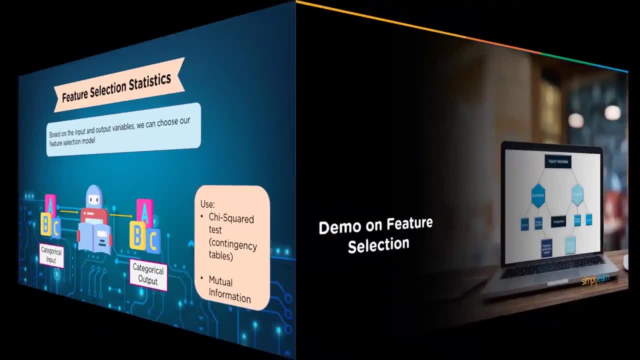 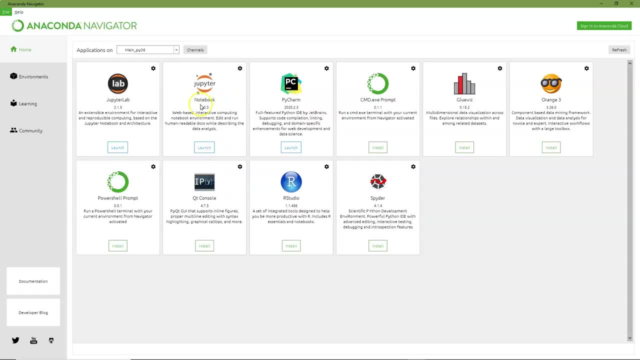 contingency tables and mutual information. Let's go ahead and take a look and see in the Python code what we're talking about here, And I'm going to go ahead and use for my IDE the Jupyter notebook in the and I always launch it out of Anaconda on here And we'll 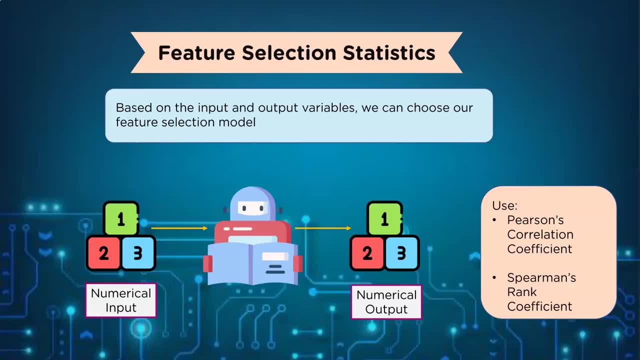 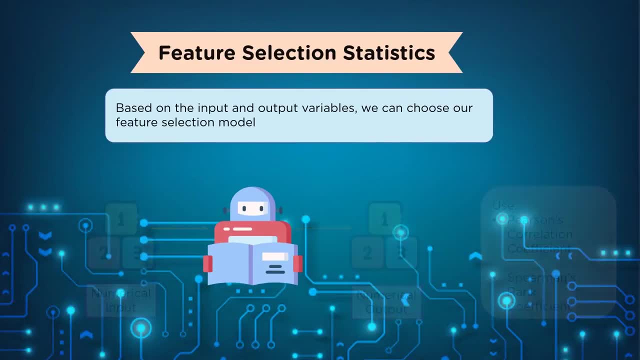 Pearson's correlation coefficient or Spearman's rank coefficient. you can then select what features you're going to feed into that specific model. You maybe have a numerical input and a categorical input. so we're going to be looking more at a NOVA correlation coefficient or Kindle's rank. 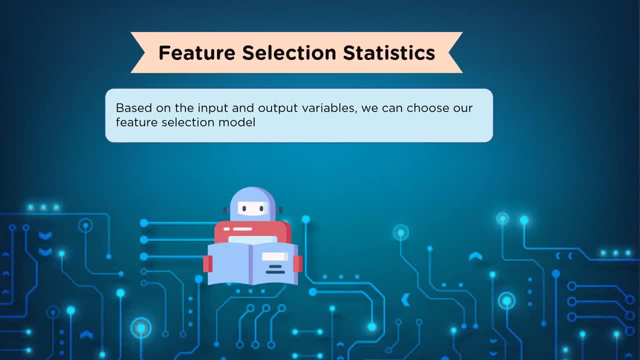 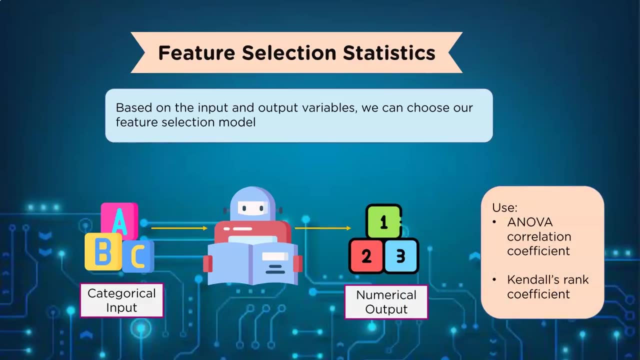 coefficient. If you have a categorical input and a numerical output, we might be looking at a NOVA correlation coefficient and Kindle's rank coefficient. So, based on the input and the output variables, we can choose our feature selection model And you can see we have categorical to. 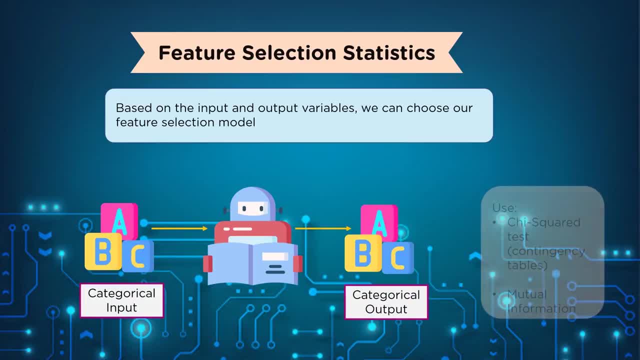 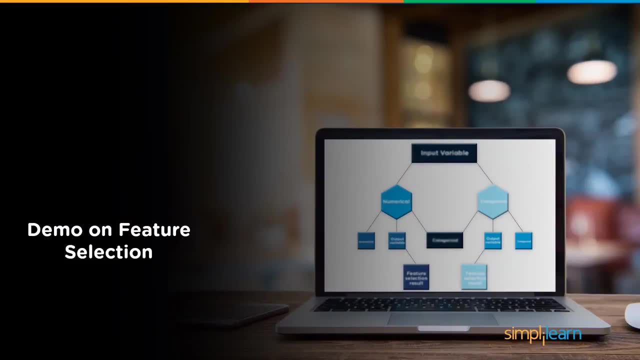 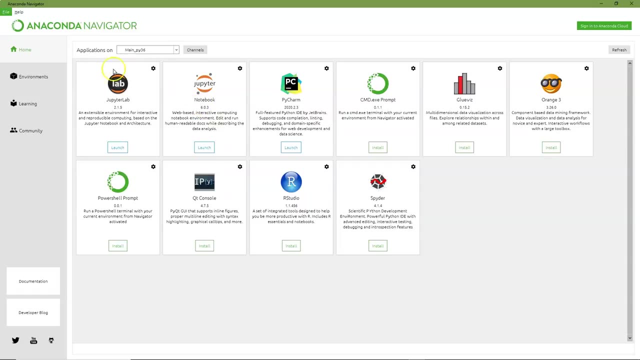 categorical. We might be looking at the chi-squared test, contingency tables and mutual information. Let's go ahead and take a look and see in the Python code what we're talking about here, And I'm going to go ahead and use for my IDE the Jupyter notebook- and I always launch it. 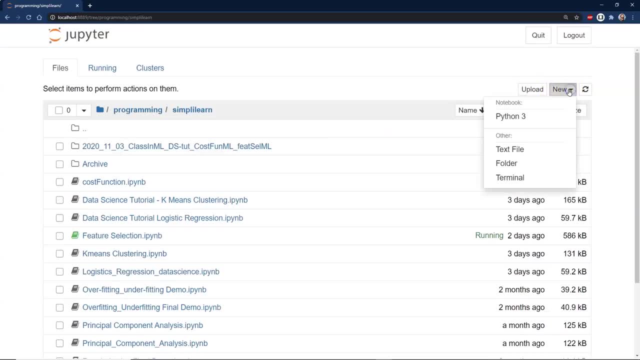 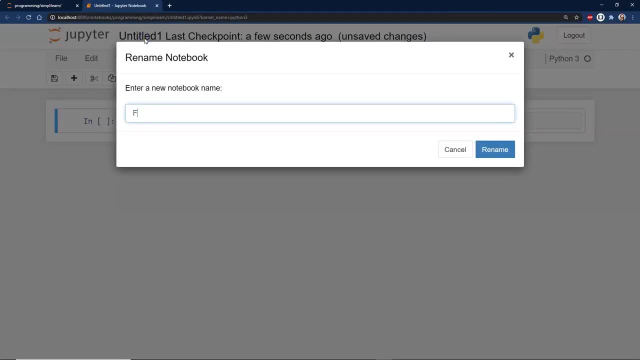 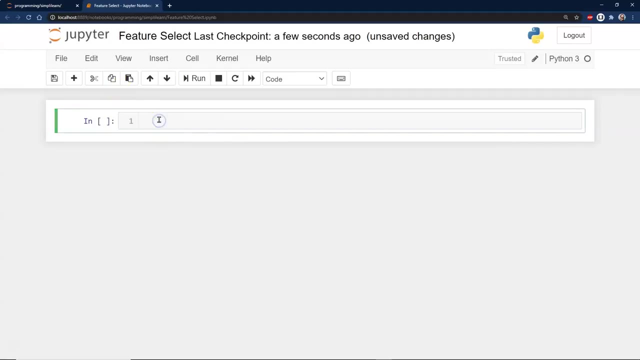 out of Anaconda And we'll go ahead and go up here and create a new Python 3 module. We'll call it feature select. Since we're in Python, we're going to be working mainly with your NumPy, your Pandas, your Matplot library. 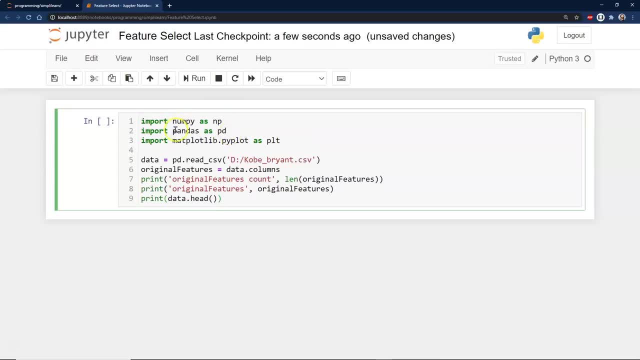 So we have our number array, our data frame setup which goes with the number array, the NumPy, the Pandas data frame, And then we want to go ahead and graph everything. So we're going to import these three modules And then we put together some data. We're going to read this in: It's a Kobe Bryant. 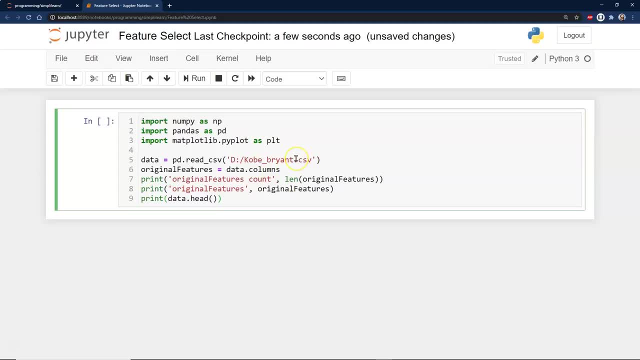 I guess he's a basketball player. Our guys in the back- we have a number of them, Guys, it's both. We have a lot of men and women, so it's probably a misnomer. Our team in the back- they have some of them have a liking for basketball and they know who Kobe Bryant is. 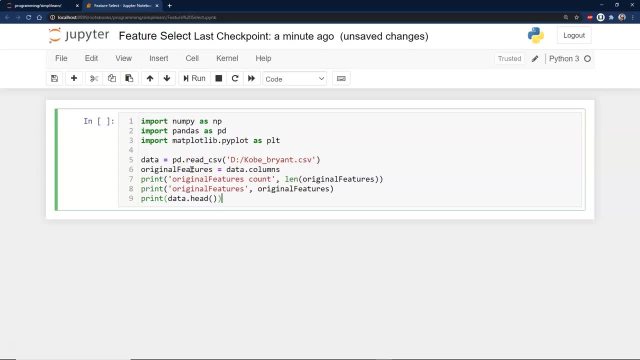 And they want to learn a little bit more about Kobe Bryant and what's going in for what. Whatever is going on with his game in basketball. So we're going to take a look at him And once we import the data, we can see what columns are available. original features count so we can see how many features there are, the length of it. 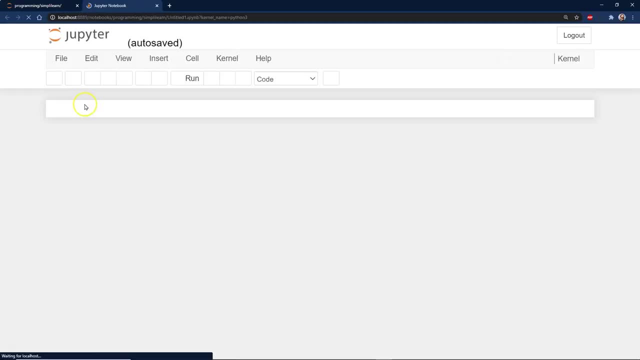 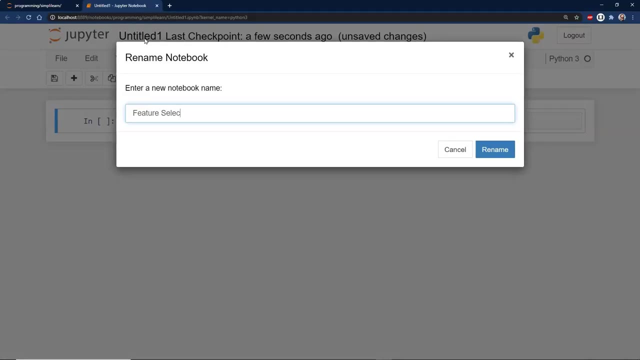 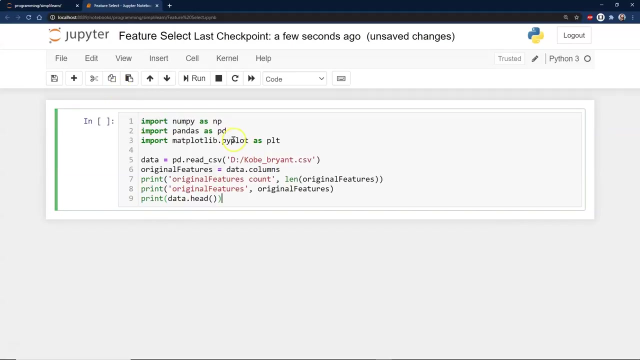 go ahead and go up here and create a new Python 3 module And we'll call it feature select. And since we're in Python, we're going to be working mainly with your numpy, your pandas, your matplot library. So we have our number array, our data frame setup, which 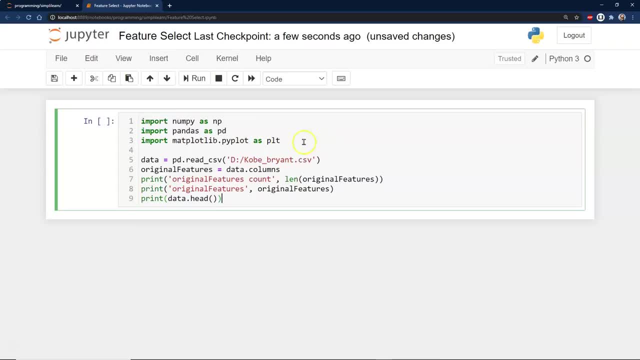 goes with the number array, the numpy, the pandas data frame, And then we want to go ahead and graph everything. So we're going to import these three modules And then we put down here some data. We're going to read this in: It's Kobe Bryant, I guess he's a. 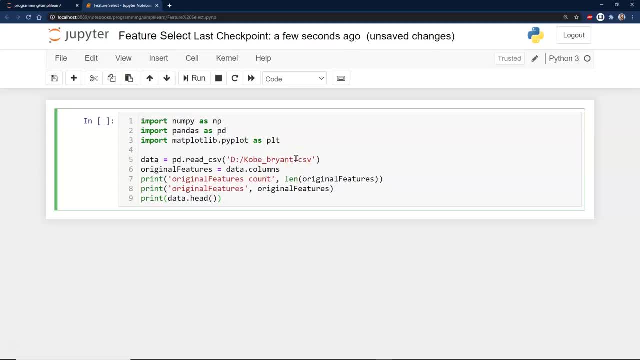 basketball player. Our guys in the back. we have a number of them, Guys, it's both. We have a lot of men and women, so it's probably a misnomer. Our team in the back. they have a. some of them have a liking for basketball and they know who Kobe Bryant is and they 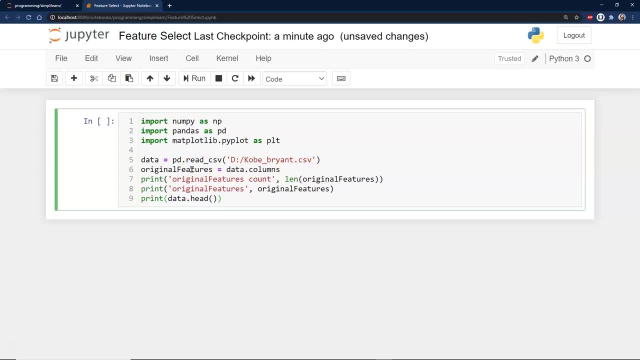 want to learn a little bit more about Kobe Bryant and what's going in for whatever's going on with his game In basketball. So we're going to take a look at him And once we import the data, we can see what columns are available. original features count, So we can see how many features there. 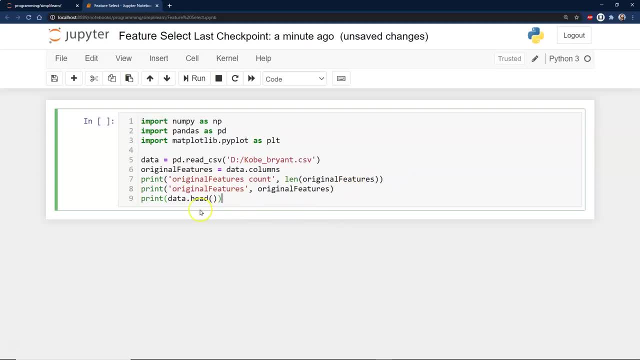 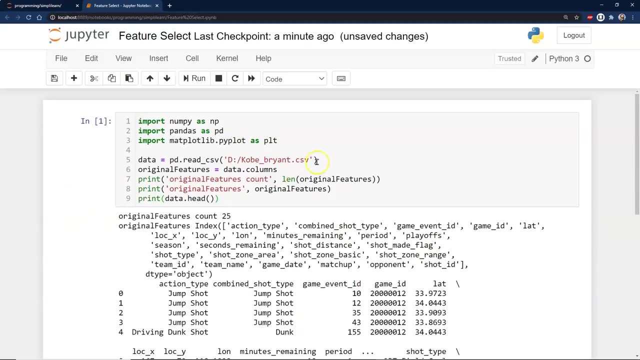 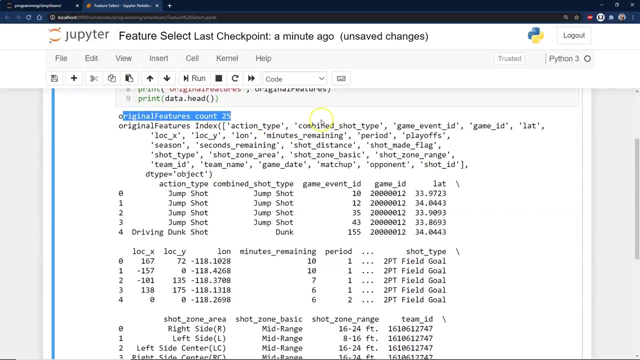 are the length of it and we'll actually have a list of them and then print just the data head, the top five rows, And so when we do this we can see from the CSV file we have 25 original features. Our original features are: your action type, combined shot. 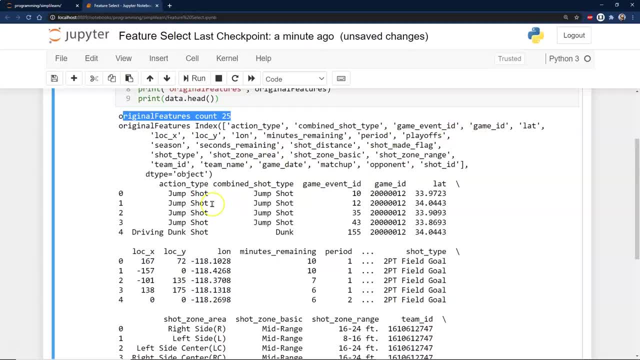 type, game, event ID and so forth. There's a lot of features in here that they recorded on all of his shots. This is what we talk about like a massive amount of data. I mean, people are sitting there and they record all this stuff and they import this stuff for. 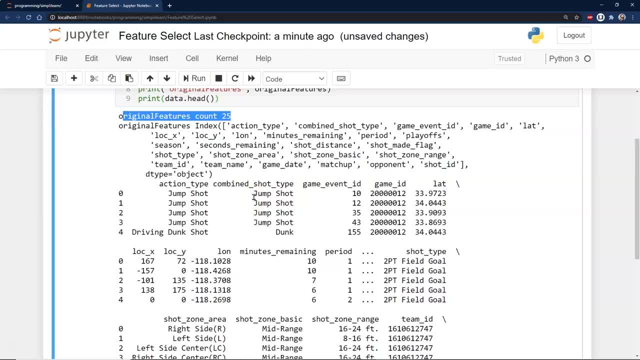 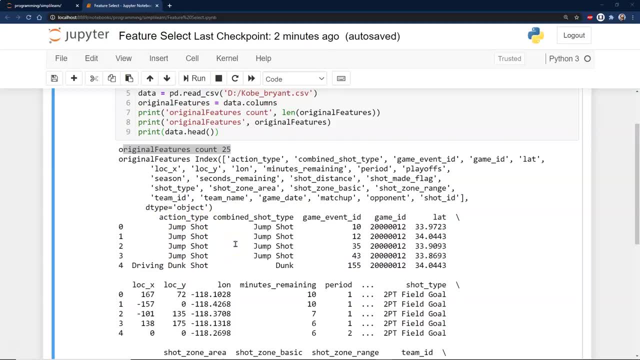 different reasons, But depending on what we want to look at. do we really want all those features? Maybe the question we're going to ask is: what's the chance of him making any one specific shot? Um, and right from the beginning, we can look at all of his shots. We can look at all of. 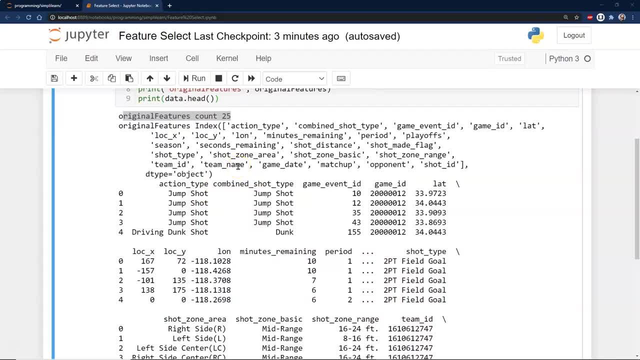 his shots. We can look at the some of these things and say team name: uh, team name, probably, I don't know, maybe it does matter because the other team might be really good at defense. Uh, game date: maybe we don't really want to look at the game date. Team ID: definitely. 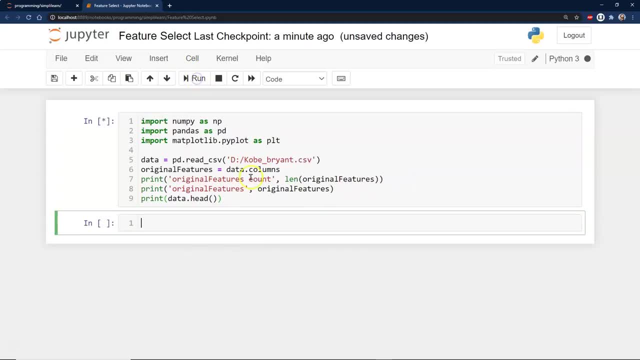 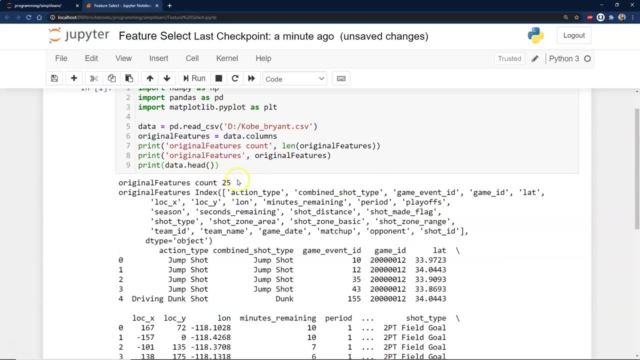 And we'll actually have a list of them and then print just the data head, the top five rows, And so when we do this we can see from the CSV file we have 25 original features. Our original features are your action. 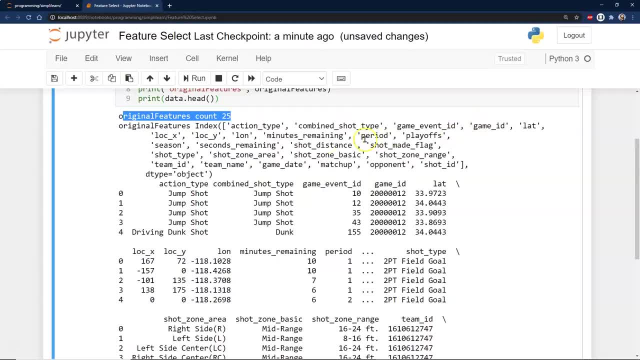 Type: combined shot type: game event ID and so forth. There's a lot of features in here that they recorded on all of his shots. This is what we talk about like a massive amount of data. I mean, people are sitting there and they record all this stuff and they import this stuff for different reasons. 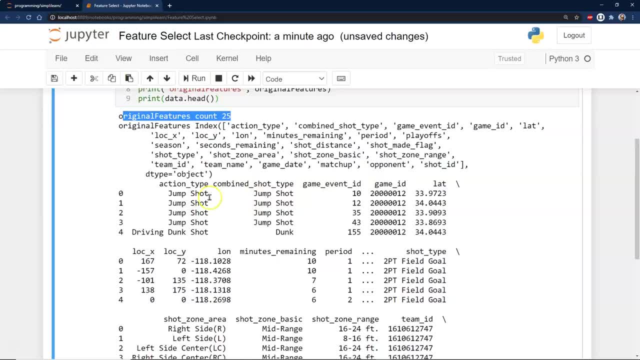 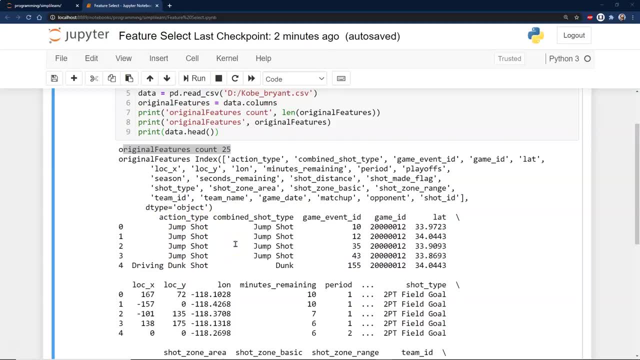 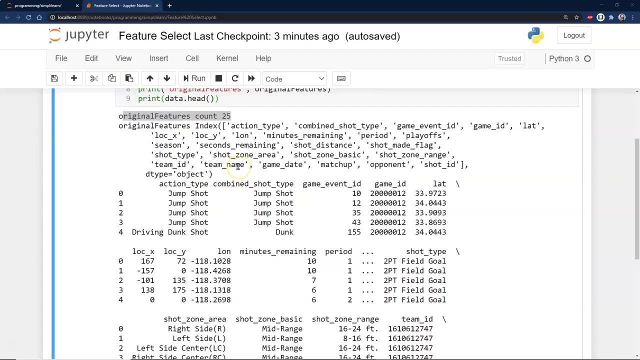 But depending on what we want to look at, do we really want all those features? Maybe the question we're going to ask is: what's the chance of him making any one specific shot? And right from the beginning we can look at the some of these things and say: team name, team name. 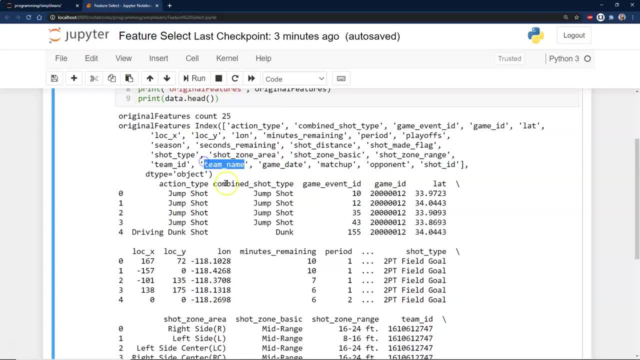 Probably. maybe it does matter because the other team might be really good at defense. game date: Maybe we don't really want to look at the game date. team ID Definitely not of importance in any of this. So we look at this. We have 25 features and some of these features just really don't matter to us. 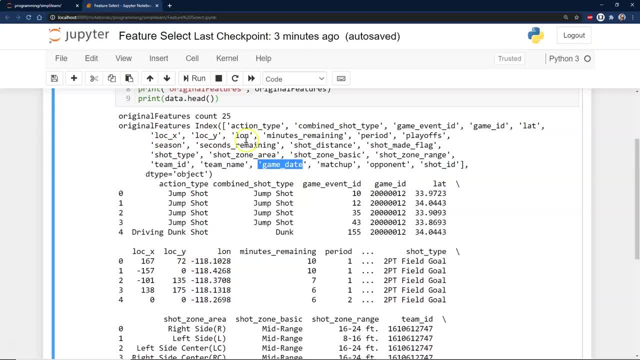 We also have location X location. Why Latitude and longitude? I'm guessing that's the same data. We've actually imported the very similar data. Maybe they're slightly zoned differently, But as far as our program we don't want to repeat data. 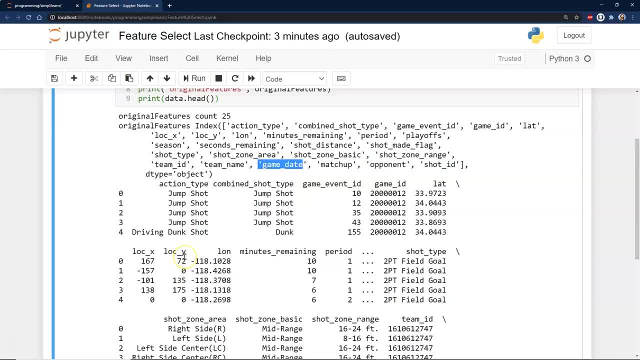 not of importance in any of this. Uh, so when we look at this, we have 25 features and some of these features just really don't matter to us. We also have location X, location Y, latitude and longitude. I'm guessing that's the same data. We've actually improved it. 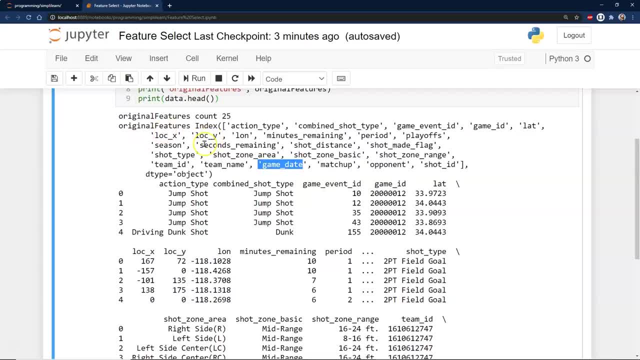 and imported the the very similar data. Maybe they're slightly zoned differently, but as far as our program, we don't want to repeat data. Some of the models, when you repeat data into them- and this is true for most models- create a huge bias. They weigh that. 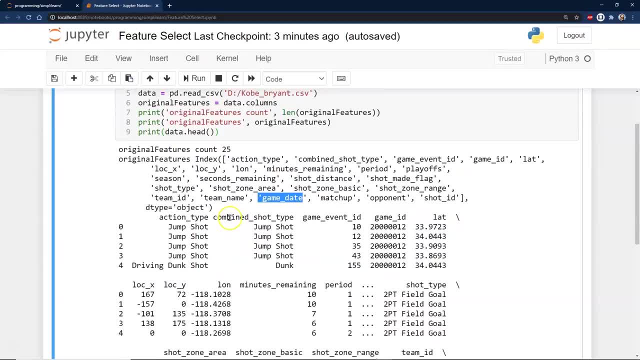 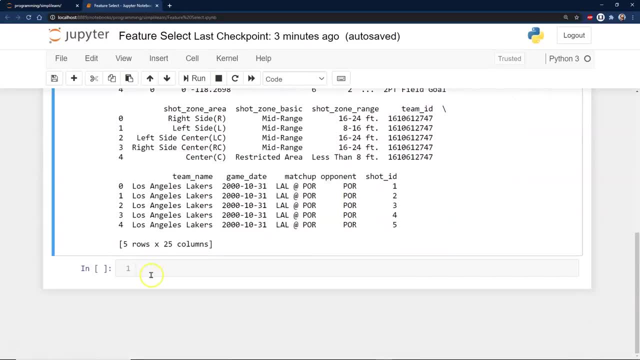 data over other data. So, just at a glance, these are the things we're looking at and we want to find out: well, how do we get this, these features, down and get rid of this bias and all these um extraneous features that we don't really want to spend time on? 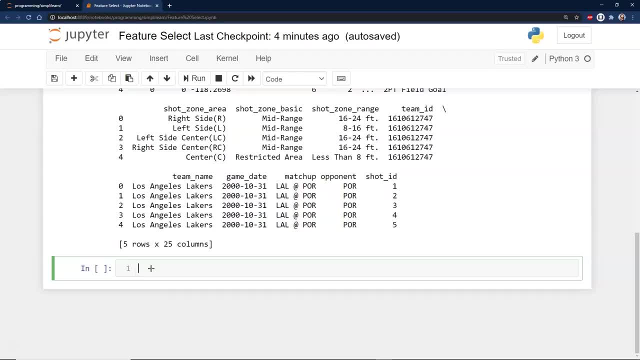 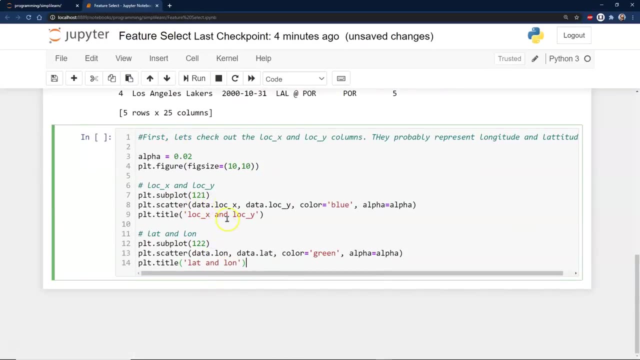 I'm running our models on and programming on And, as I pointed out, there's a location X, a location Y- latitude and longitude. Uh, let's just take a look at that and see what we're looking at here. Uh, we'll go ahead and create a plot of these and we'll just 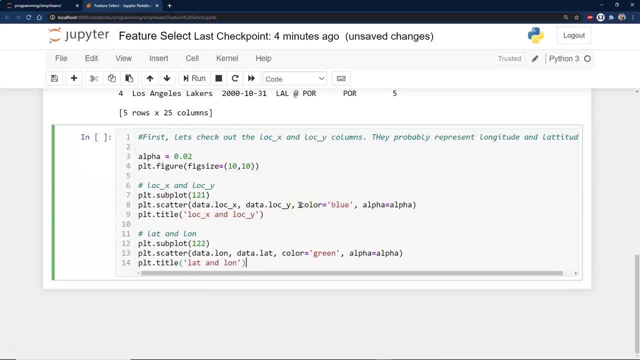 plot. uh, we'll do a scatter plot of location X and location Y and then we'll do a um, a scatter plot of um data lon, data, lat, which is probably longitude and latitude, And the scatter plot is going to actually put a little title here: location and scatter. 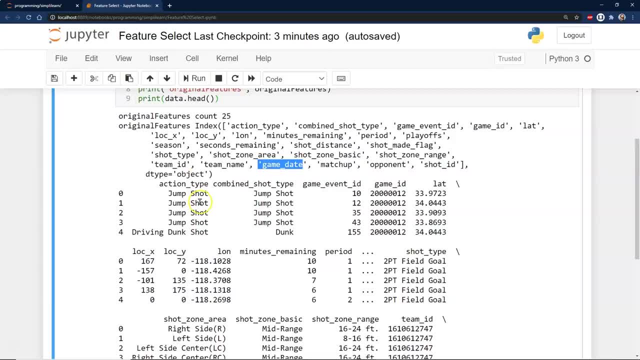 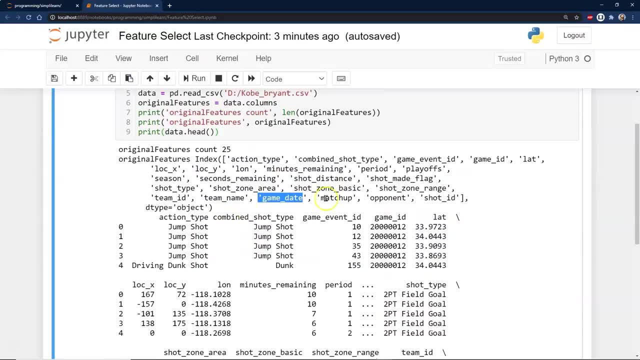 Some of the models, when you repeat data into them- and this is true for most models- create a huge bias. They weigh that data over other data. So, just at a glance, these are the things we're looking at. We want to find out: well, how do we get this, these features, down and get rid of this bias and all? 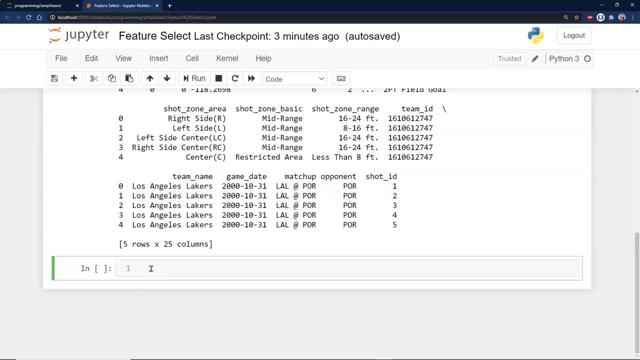 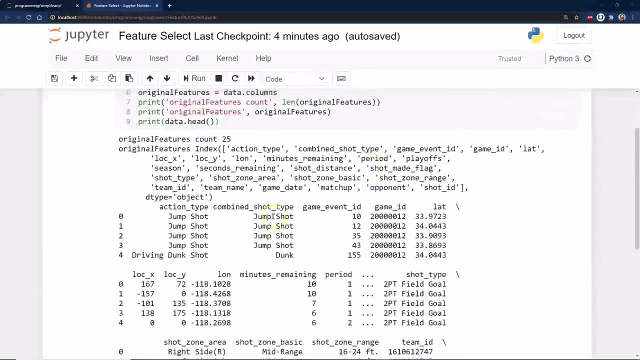 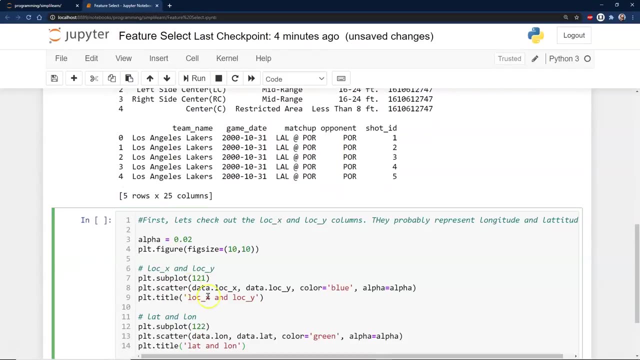 these Extraneous features that we don't really want to spend time running our models on and programming on. And, as I pointed out, there's a location, X location. Why latitude and longitude This is? take a look at that and see what we're looking at here. 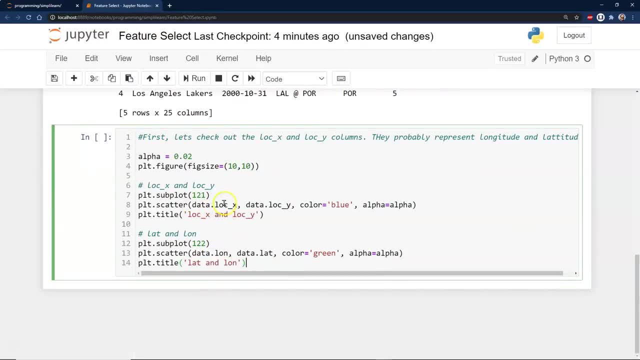 We'll go ahead and create a plot of these and we'll just plot. We'll do a scatter plot of location X and location Y and then we'll do a scatter Plot of data- long data, lat, which is probably longitude and latitude, and the scatter plot. 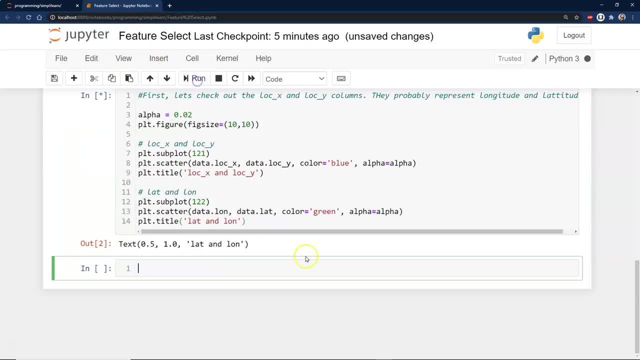 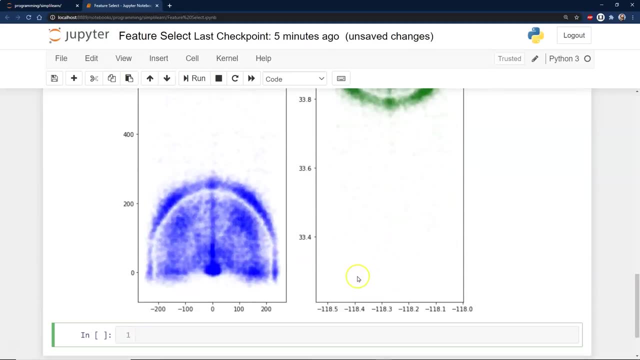 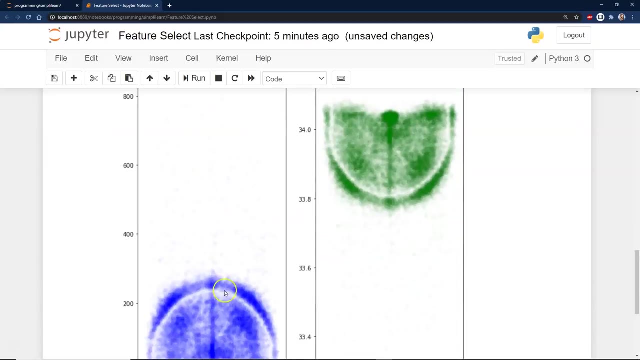 This couldn't actually put a little title here: location and scatter on there. We'll just go ahead and plot these, And when you look at this coming in, these two graphs are pretty identical, except they're flipped, And so when we look at the location from which they're shooting from, they're probably the same. 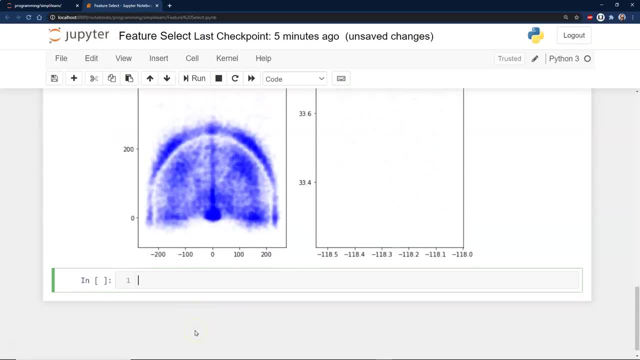 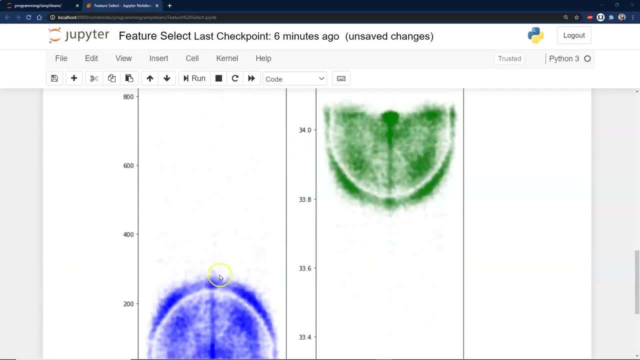 And at this point we can say, okay, we can get rid of one of these sets of data, So we don't need both X and Y and latitude and longitude, because it's the same data coming in. And as we look at this particular data- the latitude, longitude- we might also ask: 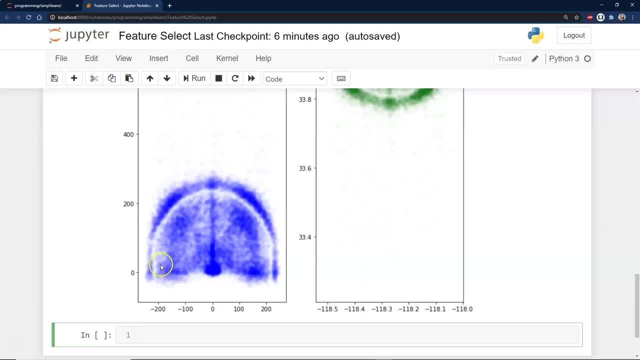 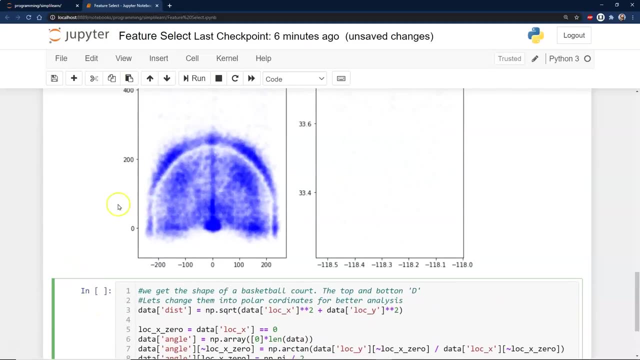 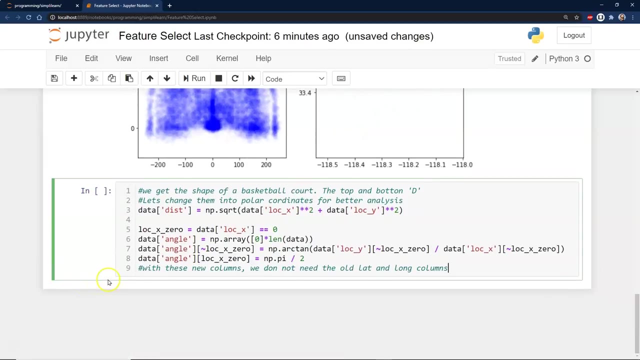 does it really make a difference which side of the court you're on, Whether you're on the left side or the right side, And so we might go ahead and explore. instead of looking at this as X, Y, we might look at it as a distance and an angle, and we can easily compute that. 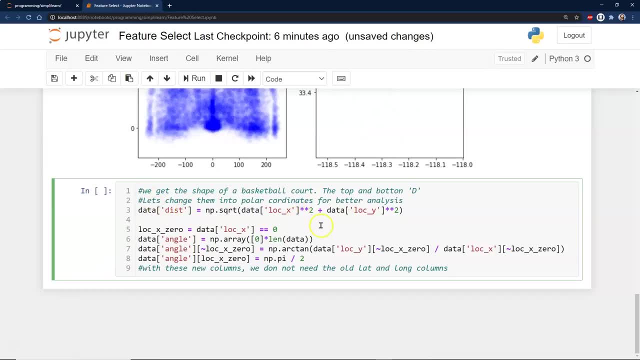 Then you can see, we can create our data. distance equals the location X plus the location Y squared. standard Euclidean geometry or triangular geometry, Hypotenuse squared equals the each side squared. And then, once we've done that, we can also compute the angle. 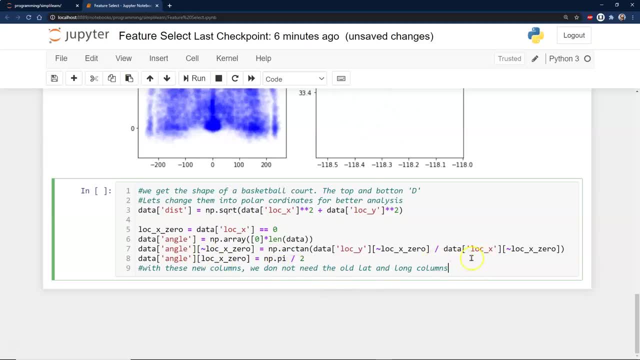 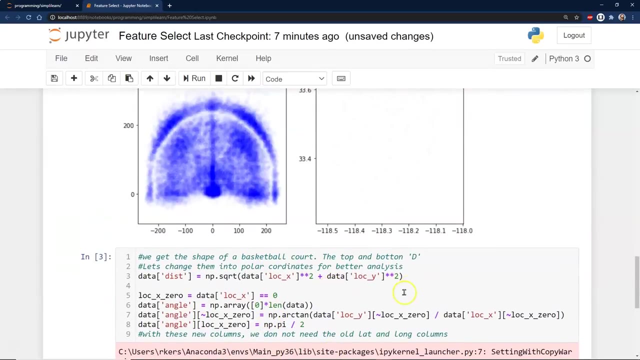 So the data angle is based on the arc tangent and so forth on here. So this is all this is is we're just going to compute the angle here and then set that up Pi over two to get our angle And we'll go ahead and run that and you'll see some errors run come up. 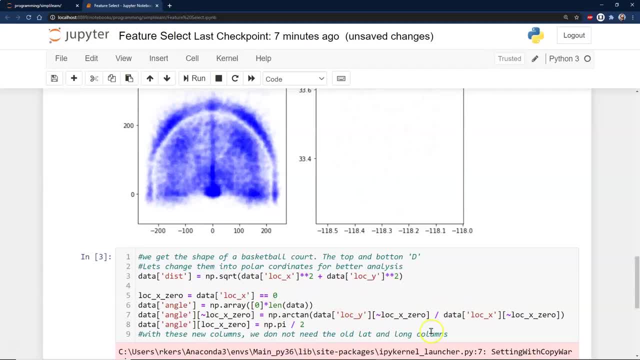 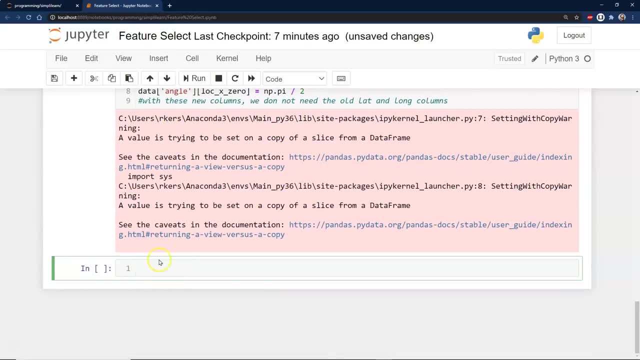 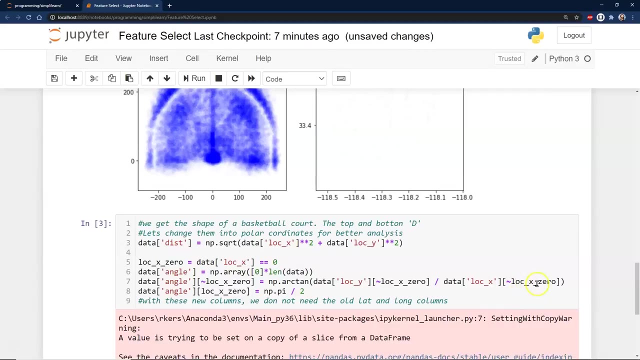 And that's because when we took slices over here, we took a slice of a slice. There's ways to fix that, but it's really not important for this example. So if you do see that, you want to start looking up here, for, instead of data, location X of, not location X, zero. 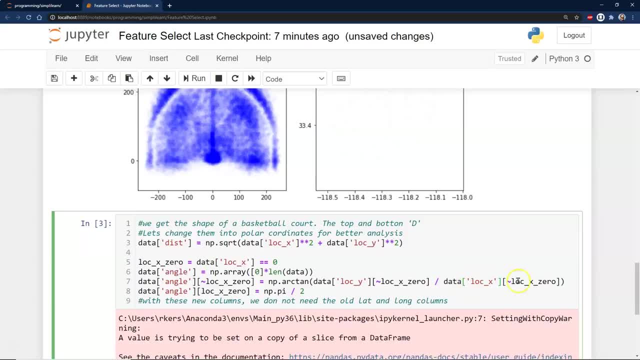 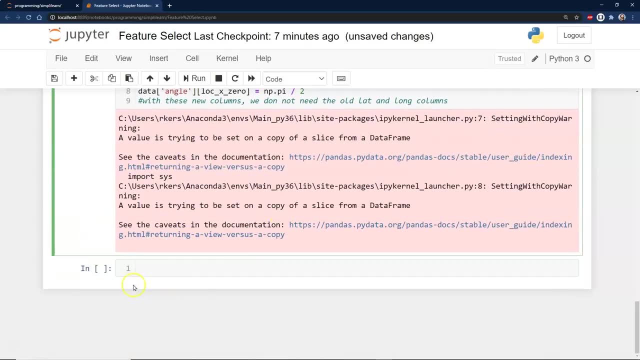 This would be like. I believe the term is eye dot, eye location. If this was, yeah, this is in pandas, So there's different things in there, but for this it doesn't really matter. These are just warnings, That's all they are. 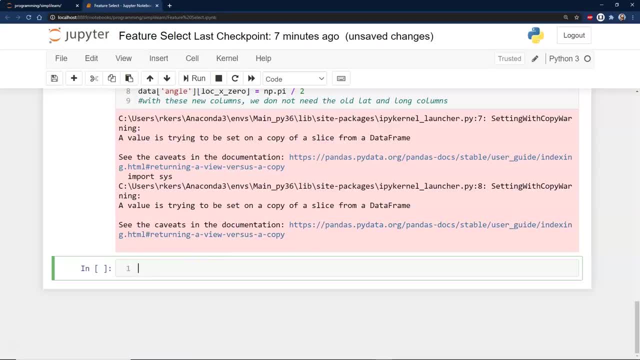 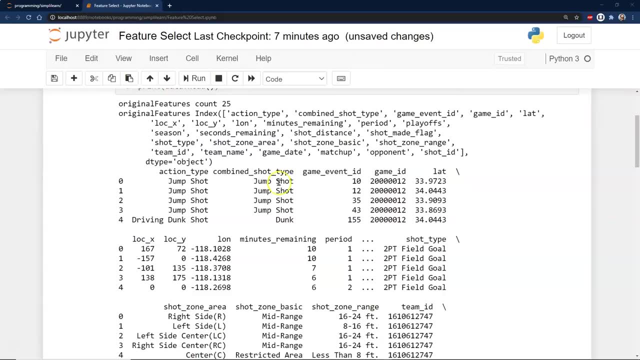 And then let's combine our remaining minutes and seconds column into one. There's another one, So, if you remember, up here we're trying to get rid of these columns. Do we really need? let me see if I can find it on here. 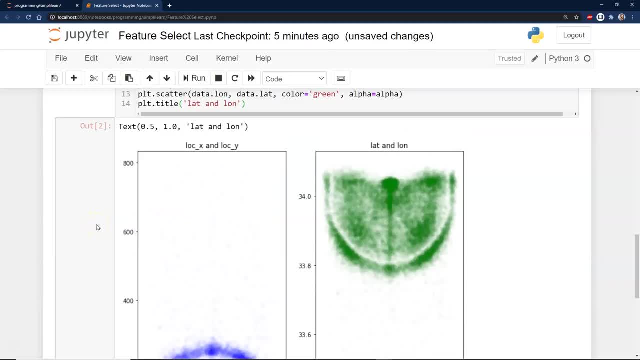 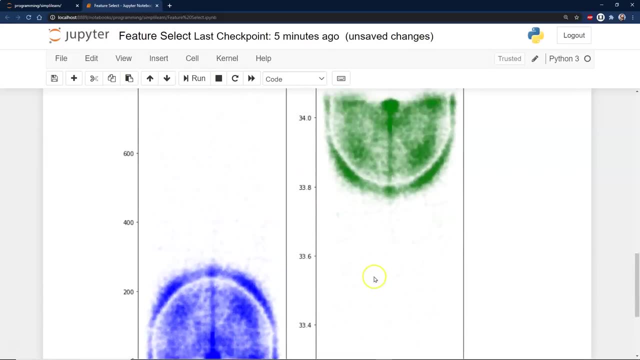 on there And we'll just go ahead and plot these. And when you look at this, uh, coming in, these two graphs are pretty identical, except they're flipped, And so when we look at the location from which they're shooting from, they're probably the same. And at this, 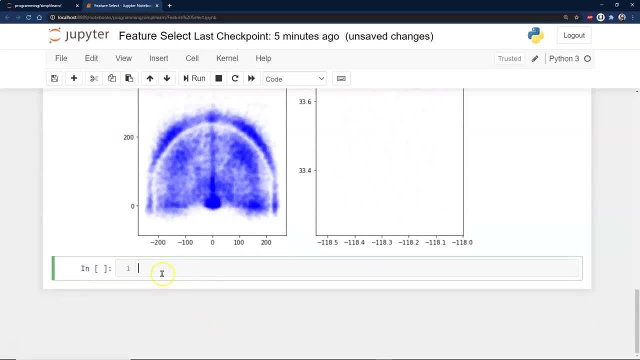 point we can say, okay, we can get rid of one of these sets of data, So we don't need both X and Y and latitude and longitude, because it's the same data coming in. And as we look at this particular data- the latitude, longitude, uh, we might also ask: 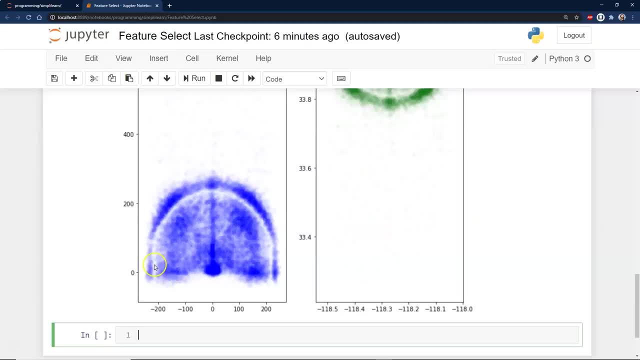 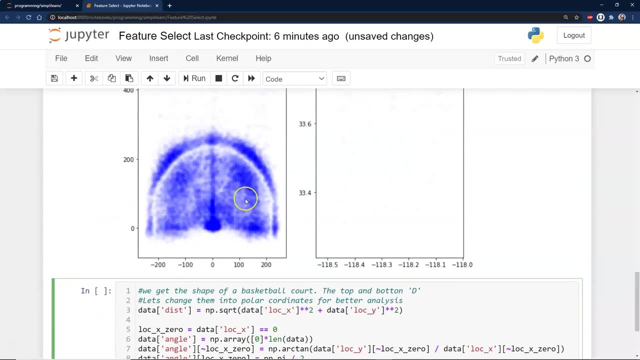 does it really make a difference which side of the court you're on, uh, whether you're on the left side or the right side, And so we might go ahead and explore. um, instead of looking at this as uh, X, Y, we might look at it as a distance and an angle, and 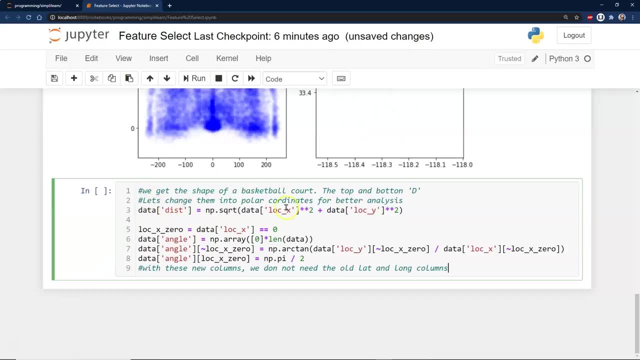 we can easily compute that And you can see, we can create our data. distance equals the location X, um plus the location Y, squared. Okay, Standard uh, Euclidean geometry or triangular geometry, hypotenuse squared equals the each side squared. And then, uh, once we've done that, uh, we can also compute the angle. Uh. 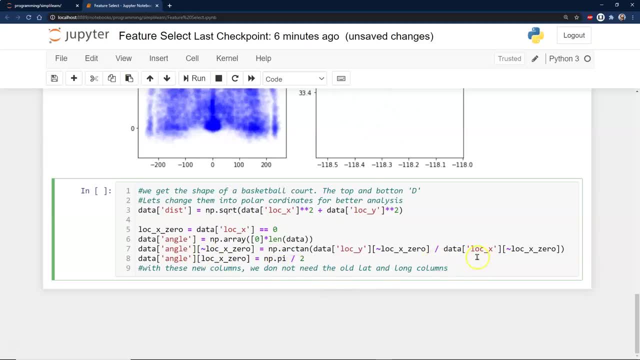 so the data angle is based on the arc tangent, uh and so forth on here. So this is all this is is we're just going to compute the angle here and then set that up- uh pi over two to get our angle. 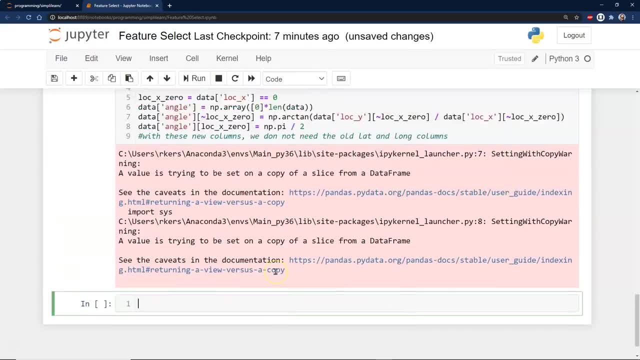 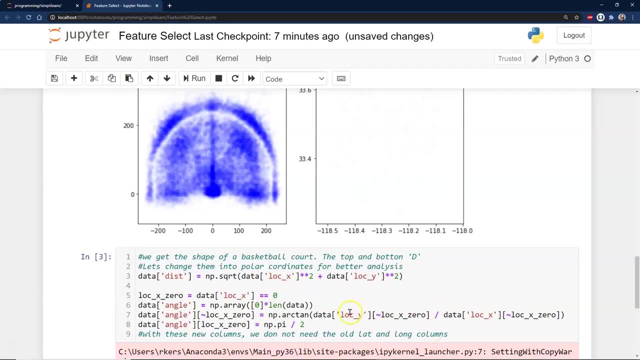 And we'll go ahead and run that And you'll see some errors run come up, And that's because when we took slices over here, we took a slice of a slice. Um, there's ways to fix that, but it's really not important. 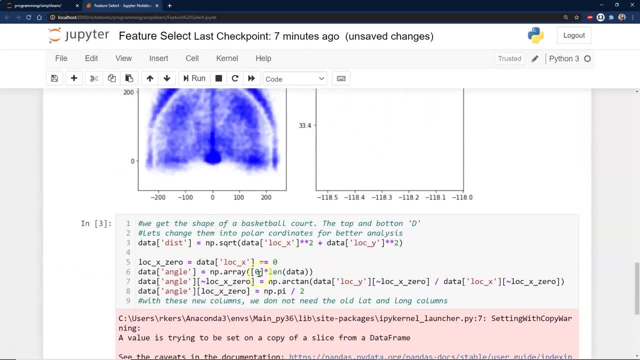 for this example: Uh. so if you do see that you want to start looking up here for um, instead of data, location X of uh, not location X zero, this would be like um- I believe the term is ILO- dot I location. 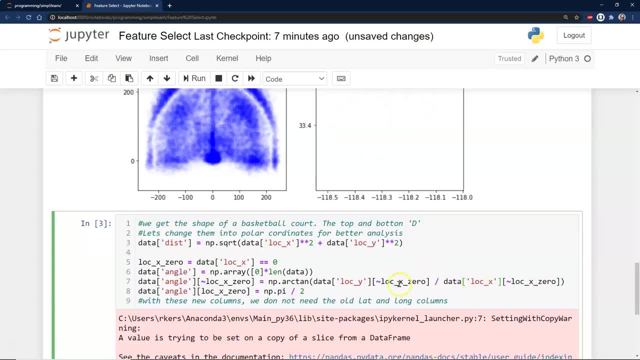 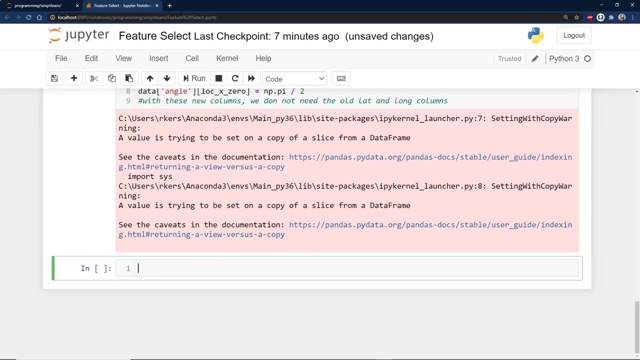 Uh, if this was, yeah, this is interesting. Okay, Yeah, I haven't had some problems with this, Okay. Okay, Let's go to the document layer. Uh, let's go to the document layer. Okay, Uh, and this one here is: um, it looks pretty good. 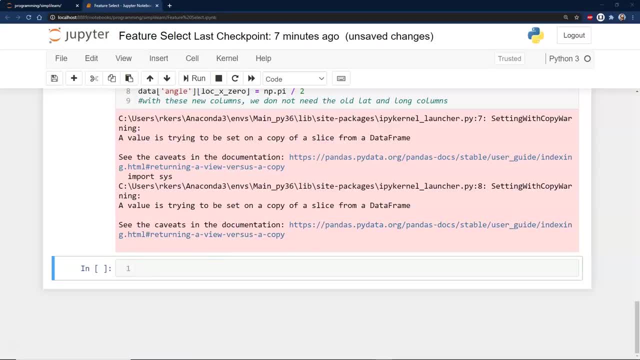 Okay, I'm going to write uh functions here. Oh, uh, I need to do this. I want to write a function. I need to write a function to this. Uh, I've got. um, let's see. 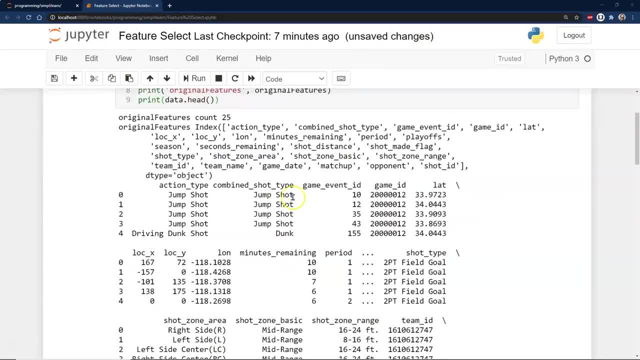 I need to write a function. I'm going to do this first in that kind of thing. I'm going to do this first in here: Uh, just delete that. Uh, just delete that. Oh, that's good. And then this one to this: 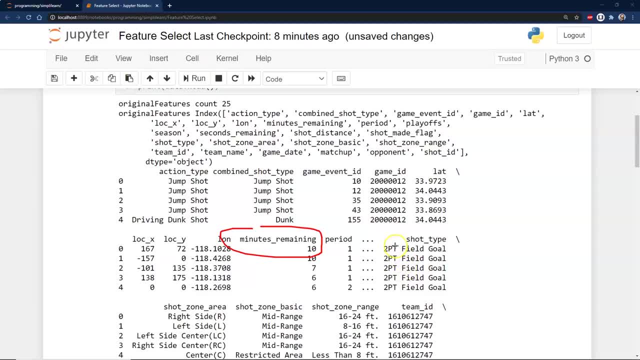 There we go. There's our minutes remaining. And then they had what was it? It was minutes remaining and seconds column. So there's also a seconds column on here. See, I can find that one. This is where it really gets kind of crazy, because here's our seconds remaining. 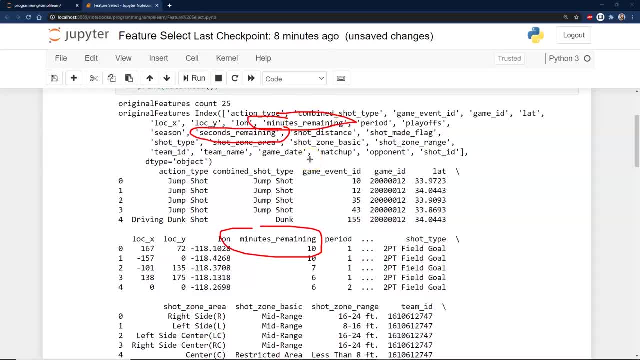 So you can see that Here's our minutes remaining. This gets crazy when you're looking at hundreds of these features and you can see that if I'm going to say write a model, that's going to predict a lot of this and I wanted to run in this case. 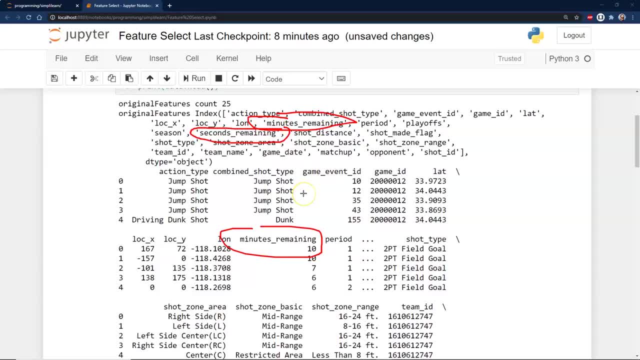 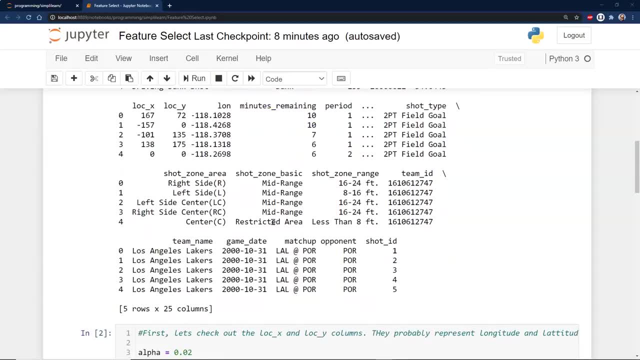 It's a basketball and how good his shots are. As the data comes in, and let's say I went around and have it run on your phone, If I'm running it across hundreds of features, it's going to just hang up on your phone where, if I can get it down to just a handful- 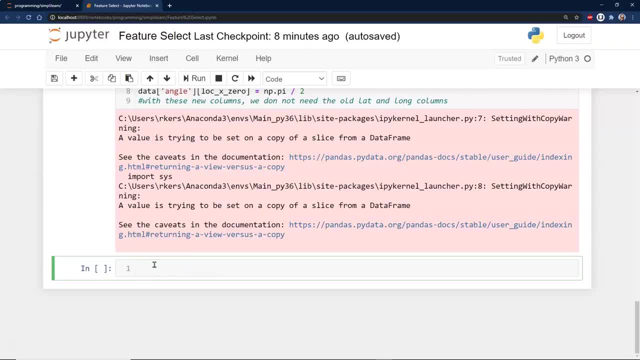 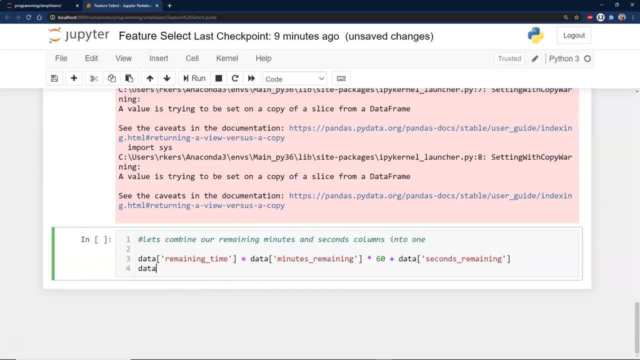 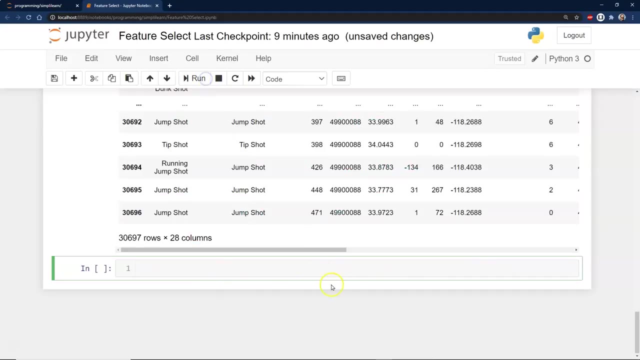 we'll actually be able to come in here and run it on a smaller device and not use up as much memory or processing power. So we'll go ahead and take data remaining time here and data minutes remaining times- 60 plus data seconds remaining, So we're just going to combine those. 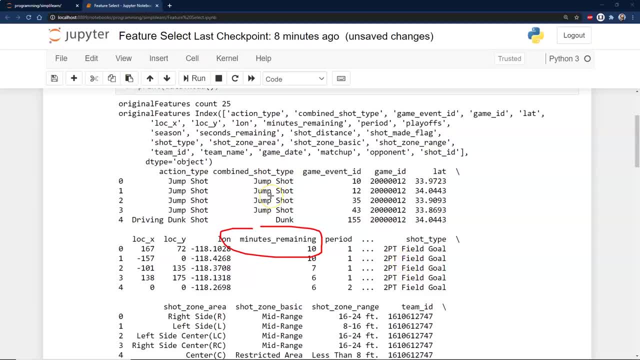 Uh, this time I'm going to have to use it for um some other functions. and then they had what was it? It was minutes remaining and seconds column. So there's also a seconds column on here. Let me see if I can find that one. 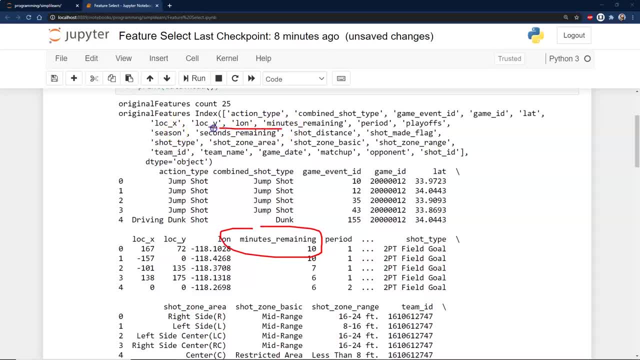 This is where it really gets kind of crazy, because here's our seconds remaining, So you can see that, and here's our minutes remaining. This gets crazy when you're looking at hundreds of these features and you can see that, if I'm going to say, write a model, 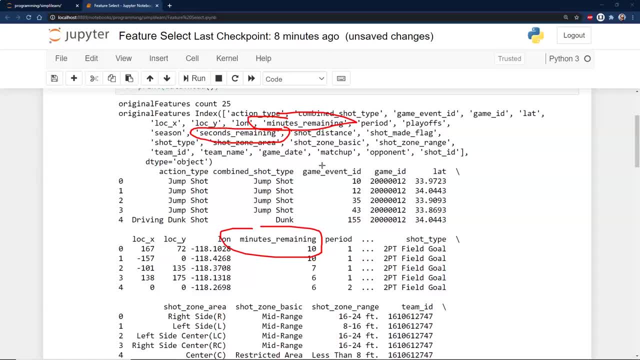 that's going to predict a lot of this and I want it to run. in this case it's a basketball, and how good his shots are. as the data comes in, Let's say: I want to have it run on your phone. 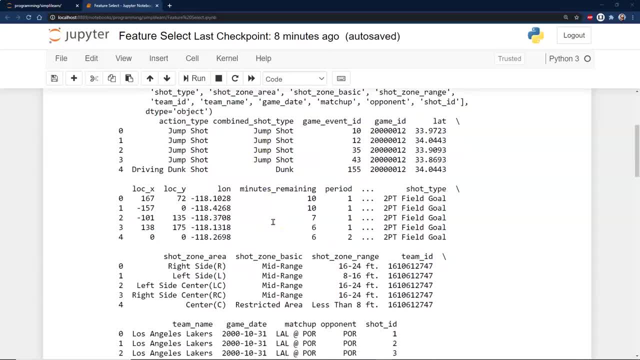 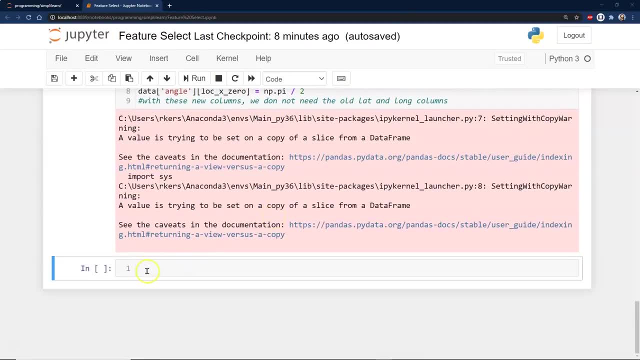 If I'm running it across hundreds of features, it's going to just hang up on your phone where, if I can get it down to just a handful, we'll actually be able to come in here and run it on a smaller device and not use up as much memory or processing power. 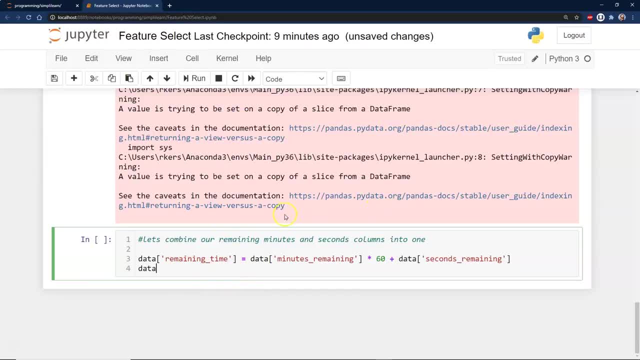 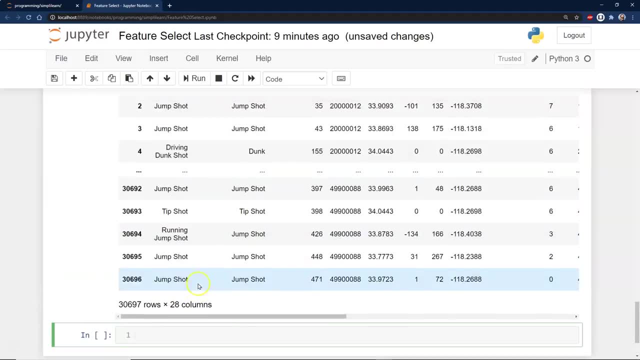 So we'll go ahead and take data remaining time here and data minutes remaining Time: 60 plus data seconds remaining. So we're just going to combine those and we'll go ahead and reprint our data so we can see what we got. 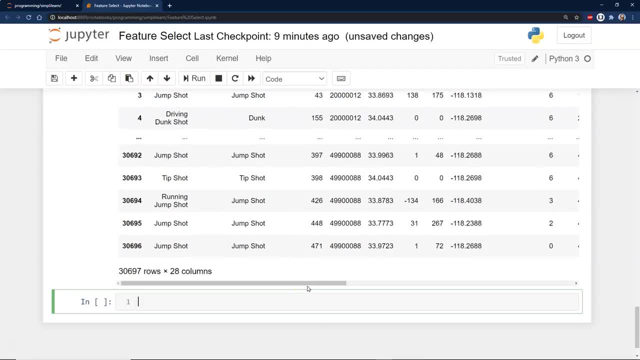 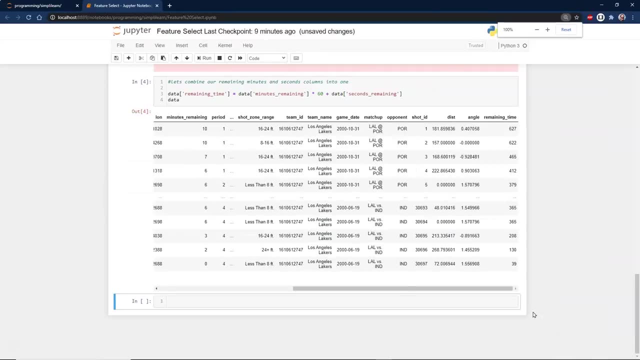 Coming across. we have our action type combined and we do this a lot. We want to take a look at Oops, I got it so zoomed in. Let me see if I can zoom out just a little bit. There we go. 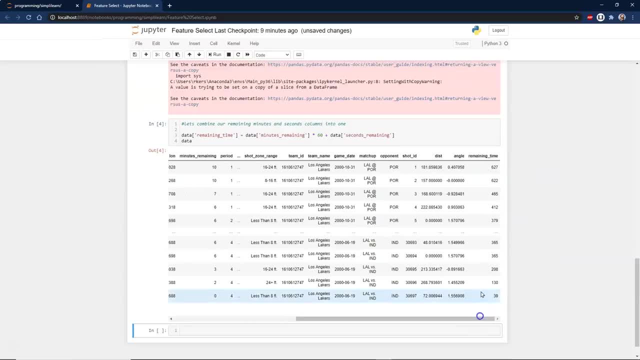 Boom. All right. so when we come up here, you can see that we now have our distance, our angle, remaining time, which is now just a number that computes both the minutes and seconds together, And we still have. We've been adding columns. 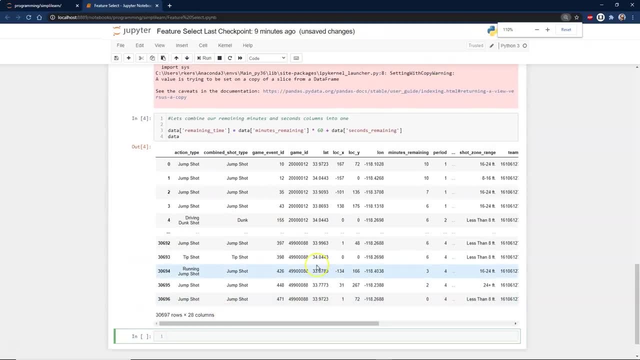 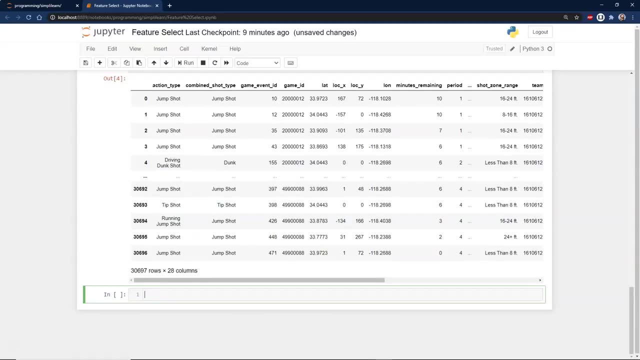 I thought you said we're supposed to subtract columns, right, We're going to delete the obsolete columns when we get to them, So we're just filtering out, and this is a filter method. We're just filtering through the things that we really don't need. 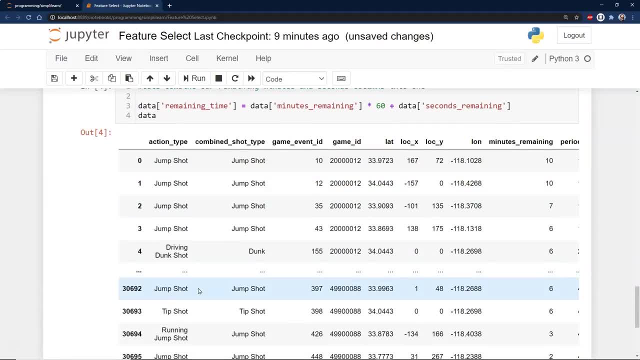 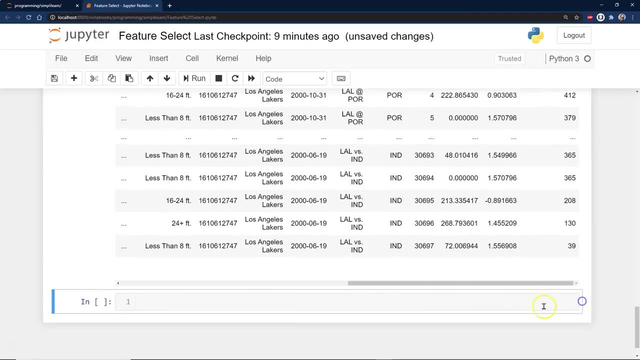 And we'll go ahead and reprint our data so we can see what we got coming across. We have our action type combined and this is we do this a lot. We want to take a look at that. I got so so zoomed in. 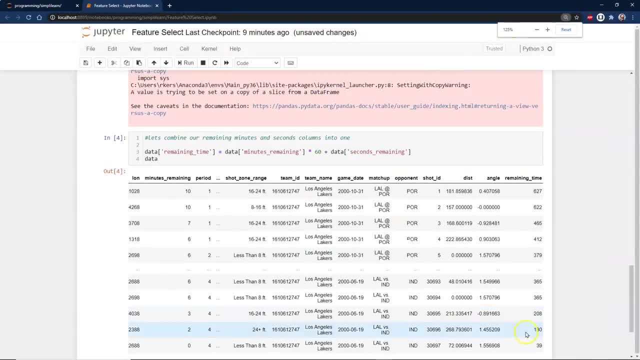 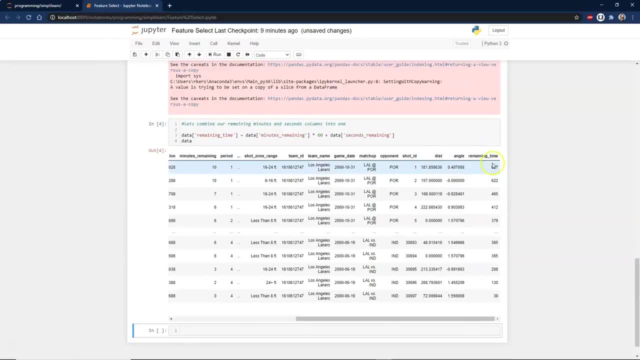 Let me see if I can zoom out just a little bit. There we go, Boom, All right. So we come up here. You can see that we now have our distance or angle remaining time, which is now just a number that computes both the minutes and seconds together. 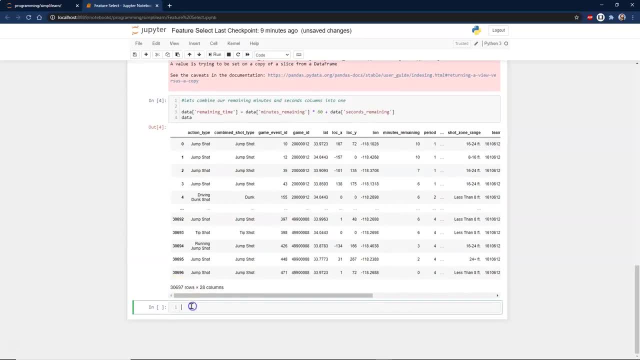 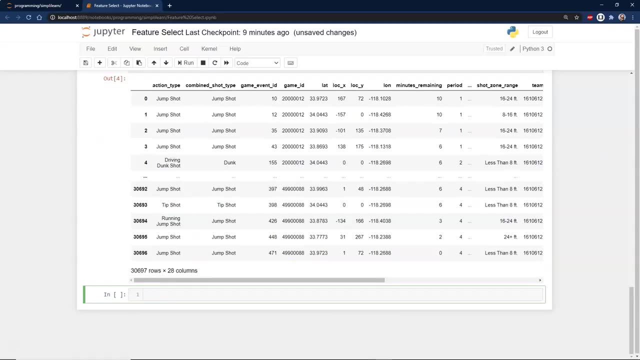 And we still have. we've been adding columns. I thought you say we're supposed to subtract columns. right, We're going to delete the obsolete columns when we get to them. So we're just filtering out And this is a filter method. 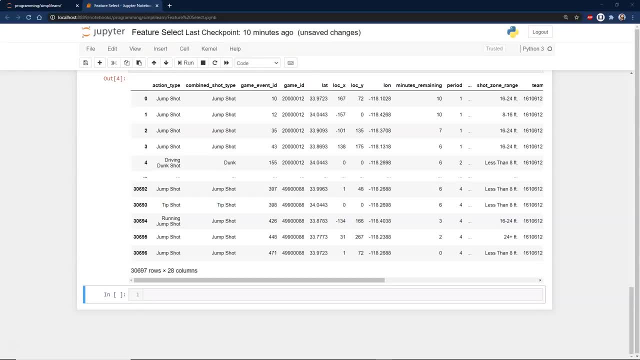 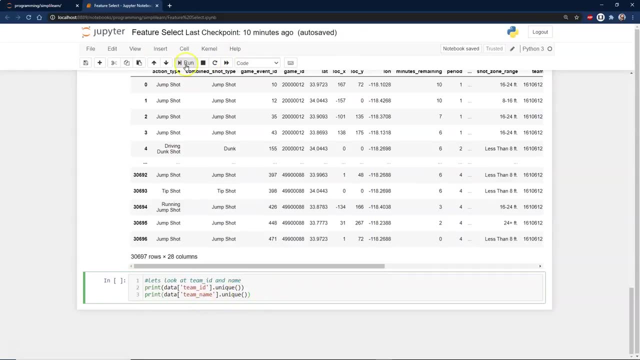 We're just filtering through the things that we really don't need, And next let's go ahead and explore team ID and team name. Let me just go ahead and run that And if you look at this, we have Los Angeles Lakers. 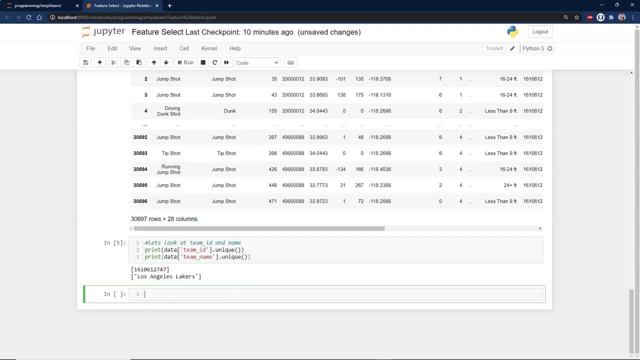 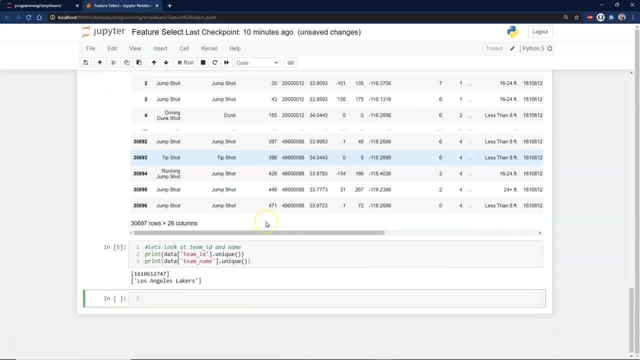 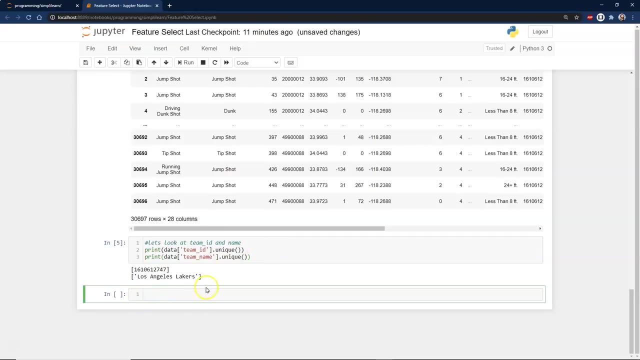 And then they have the team ID Here and they're unique. There's not- that's not really anything that's going to come up, because that's this particular athletes works for that team, So it's the same on every line. So there's another thing we can filter out on their team ID, and team name is just useless. 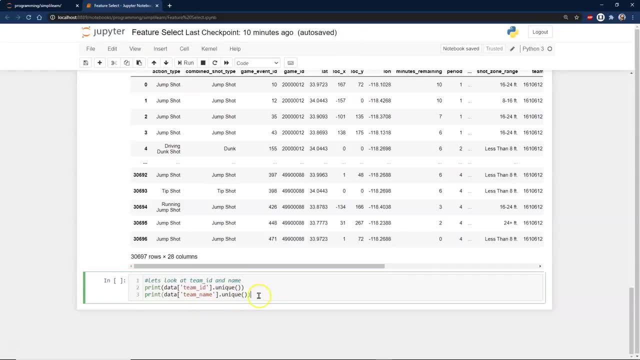 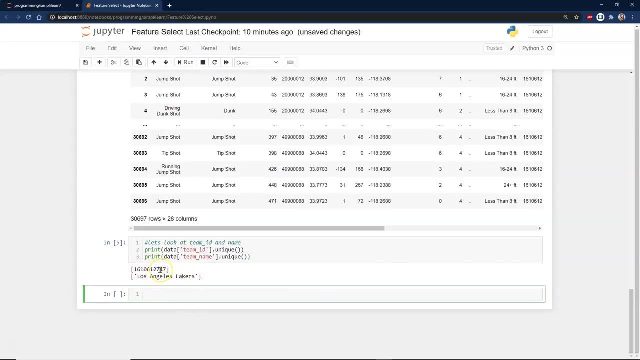 And next let's go ahead and explore team ID and team name. Let me just go ahead and run that And if you look at this, we have Los Angeles Lakers and then they have the team ID here and they're unique. 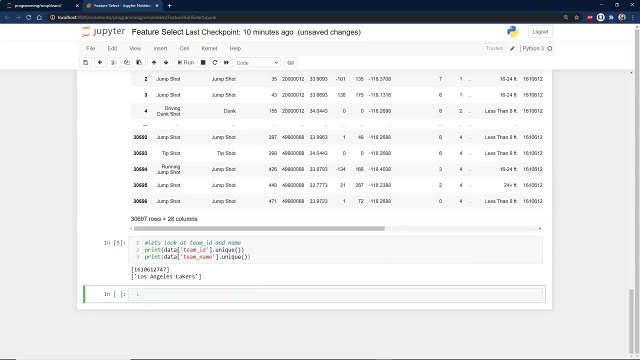 That's not really anything that's going to come up because this particular athlete works for that team, So it's the same on every line. So there's another thing we can filter out on there. Team ID and team name is just useless. 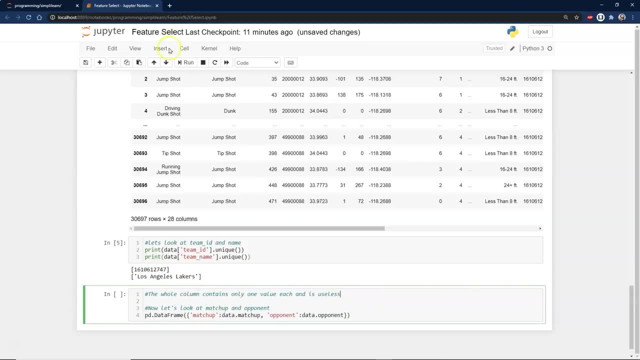 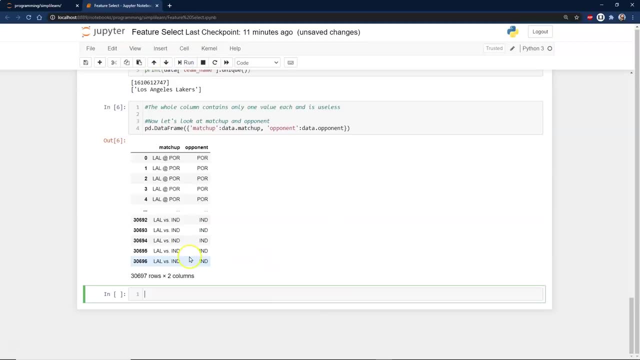 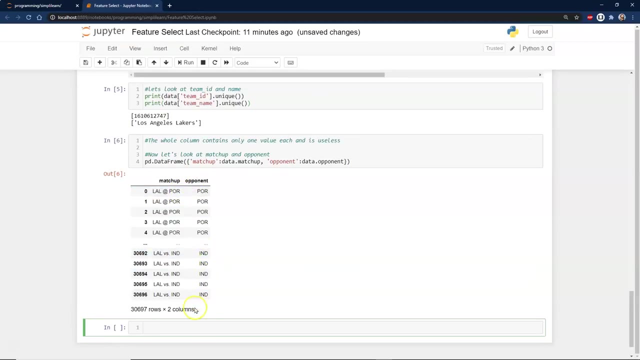 The whole column contains only one value each, and it's pretty much useless. Let's go ahead and take a look at matchup and opponent. That's an interesting one, And we see here that we have the LAL versus POR and the opponent is POR and IND. 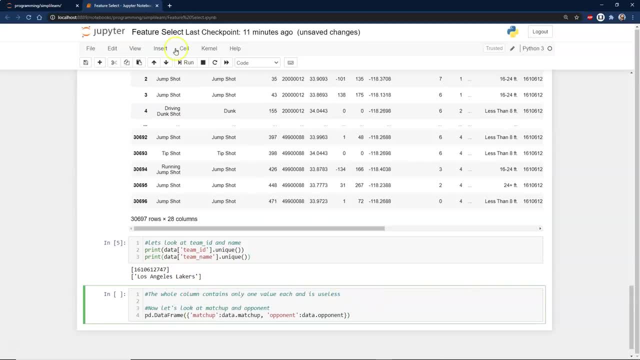 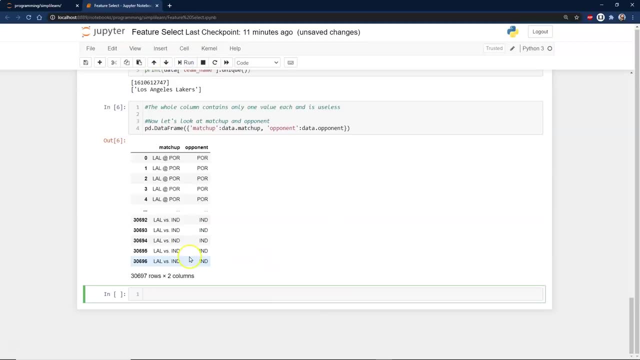 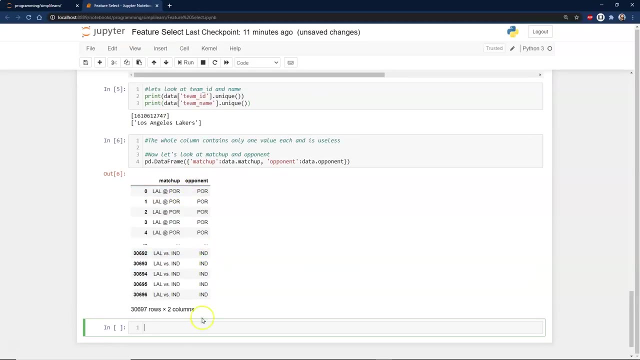 The whole column contains only one value each, and it's pretty much useless. Let's go ahead and take a look at match up and opponent. That's an interesting one, And we see here that we have The LAL versus POR and the opponent is POR and IND again. 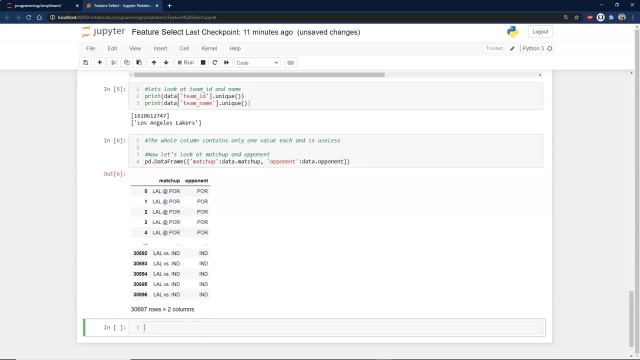 Here's a lot of duplicate information, So this basically contains the same information on here Again, we're filtering all this stuff out, And this is because we're only looking at one athlete. This might change if you're looking at multiple athletes- that kind of thing. 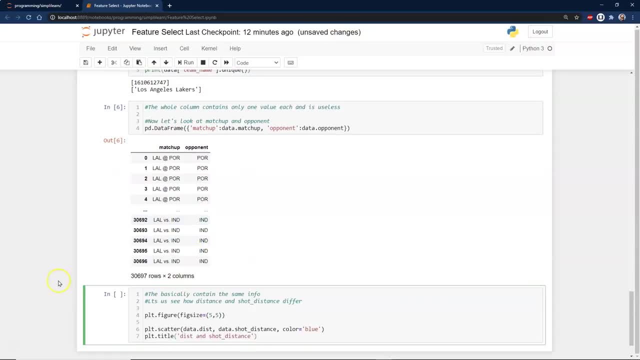 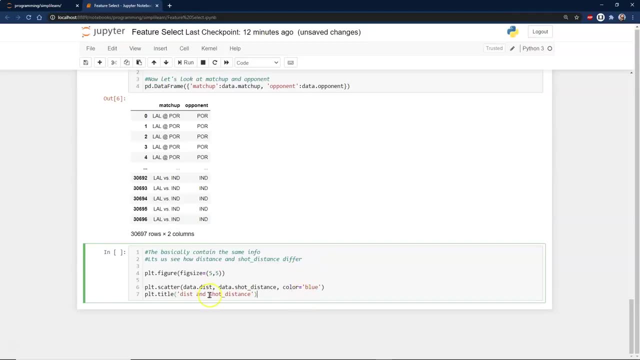 Now, these are easy to see. We might have something that looks more like this. We might have something where we're looking at The Distance which we computed and the shot distance- Are they the same thing? And what we can do is we can plot that and plot them against each other on here. 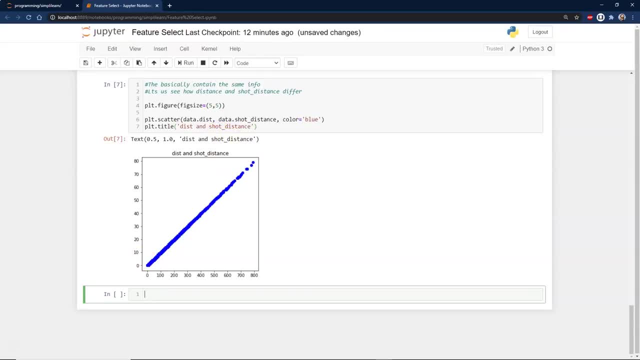 And we see it just draws a nice straight line. And so again we're looking at the same information. So again we're repeating stuff and we really don't want to be running our model on repeat information on here. So again it contains the same information. 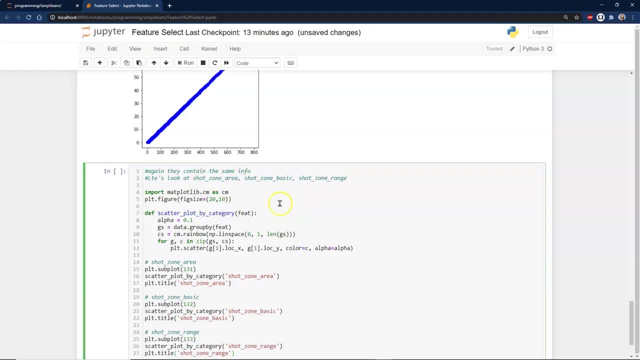 So now let's look at the shot zone: area, Shot zone, basic, shot zone range. So now we're looking at the zones and what does that mean? And we'll go ahead and do this also in a scatter plot. In this case, we're going to just create three of these side by side. 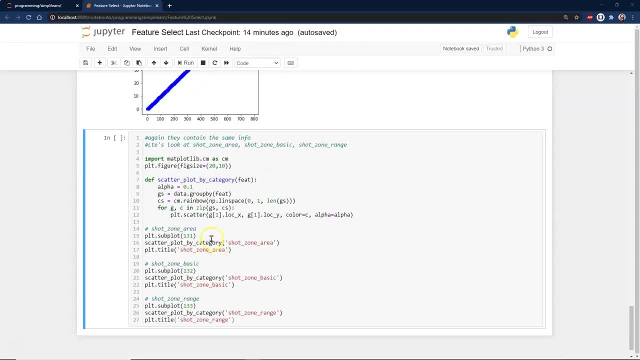 So we're going to create our plot, figure side 20 by 10.. And then we're going to define our scatter plot by category feature, And we're going to do each one set up on here, Give it a slightly different color, And so our shot zone area is going to be plot. 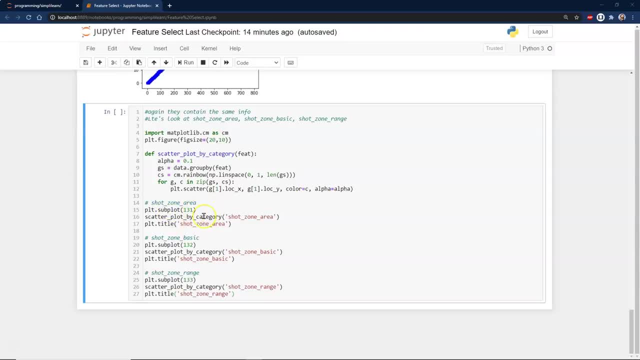 Subplot 131. scattered 131 is how that's read, by the way, Meaning that it's number one. We have three across and this is the first one down, So 111, our scatter plot by category, is going to be the shot zone area. 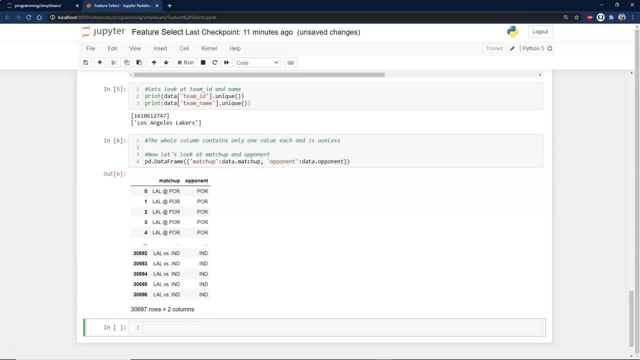 Again, here's a lot of duplicate information, So this basically contains the same information on here Again, we're filtering all this stuff out, and this is because we're only looking at one athlete. This might change if you're looking at multiple athletes, that kind of thing. 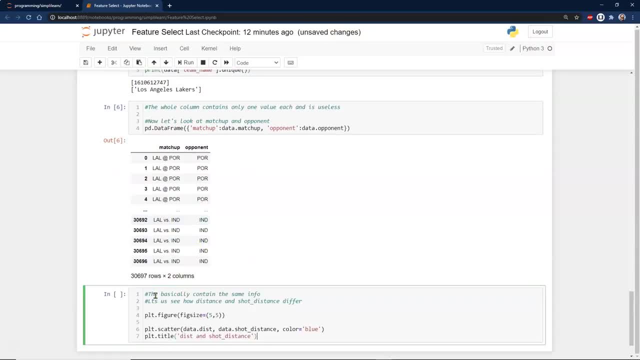 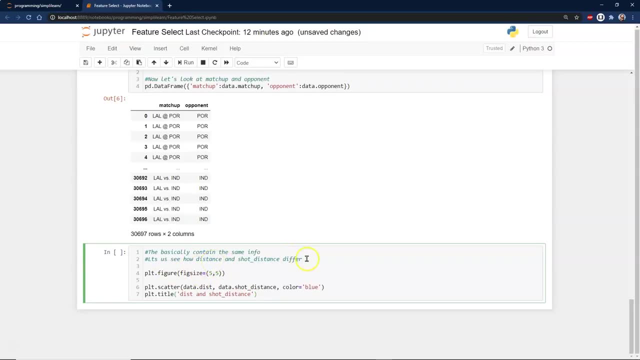 Now, these are easy to see, but we might have something that looks more like this. We might have something where we're looking at the distance which we computed and the shot distance- Are they the same thing? And what we can do is we can plot that. 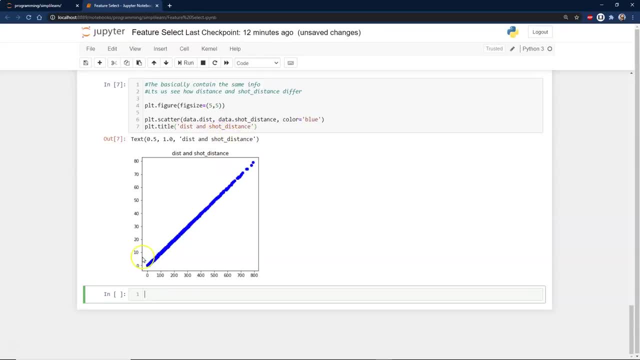 and plot them against each other on here and we see it just draws a nice straight line. And so again we're looking at the same information, So again we're repeating stuff and we really don't want to be running our model on repeat information on here. 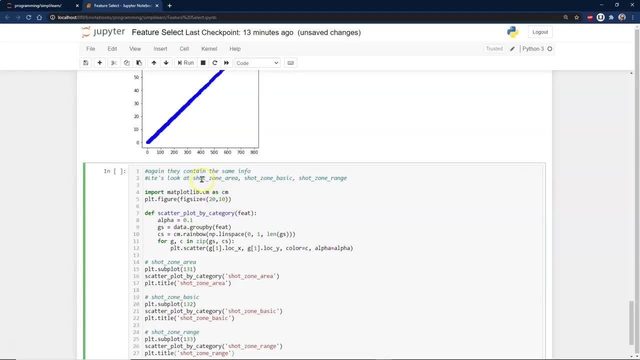 So again, it contains the same information. So now let's look at the shot zone area, shot zone basic, shot zone range. So now we're looking at the zones and what does that mean? And we'll go ahead and do this also in a scatter plot. 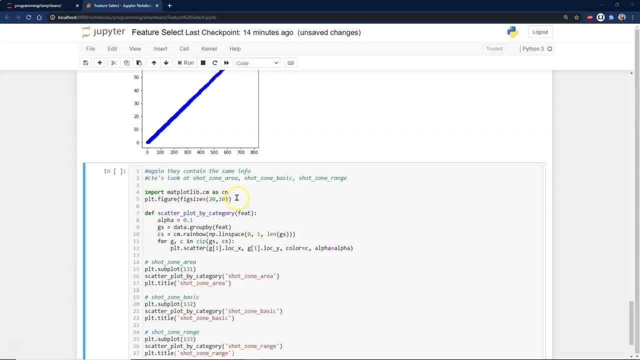 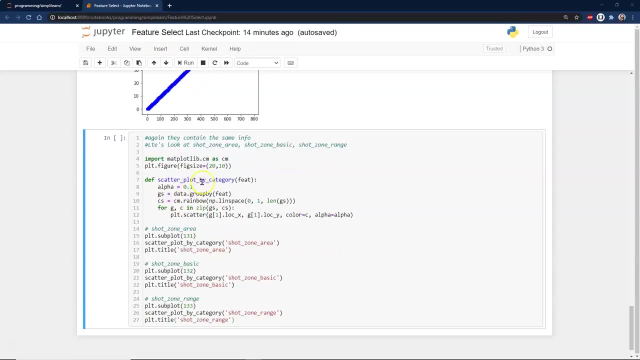 In this case we're going to just create three of these side by side. So we're going to create our plot figure side 20 by 10, and then we're going to define our scatter plot by category feature and we're going to do each one set up on here. 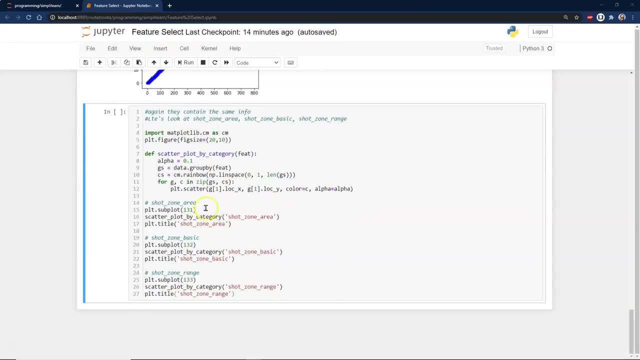 give it a slightly different color, And so our shot zone area is going to be plot subplot 131, scatter 131 is how that's read, by the way, meaning that it's number one. we have three across and this is the first one down, so 111.. 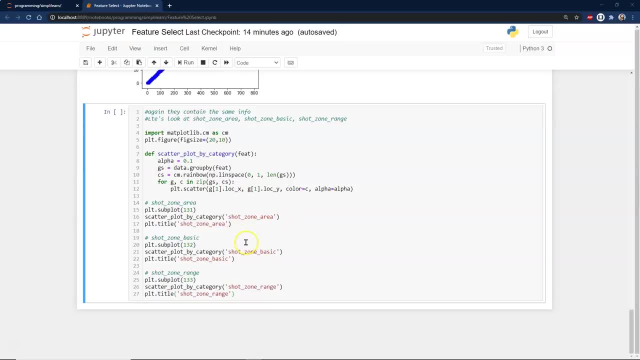 Our scatter plot by category is going to be the shot zone area. We're going to plot that and then we're going to do the shot zone basic and then the shot zone range and each just push them through our definition. So each of those areas go through and you'll see 131, 132, 133.. 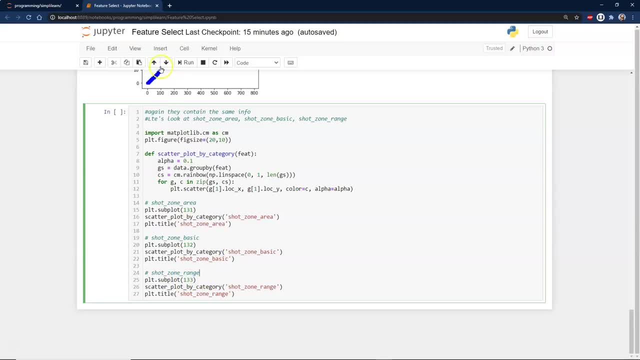 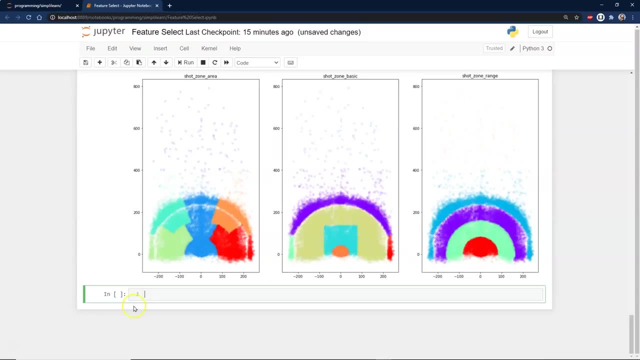 Again, it's a one by three set up and then it's just a place on each one, And so we look at this. we can see that these shots, they map out the same. So it's very, again, redundant information. 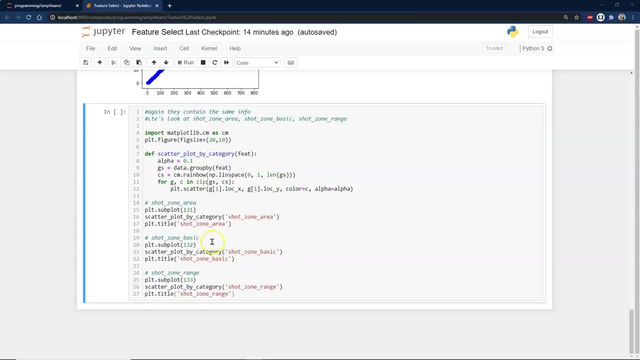 We're going to plot that and then we're going to do the shot zone basic and then the shot zone range and each just push them through our definition. So each of those areas go through and you'll see 131.. 132, 133. 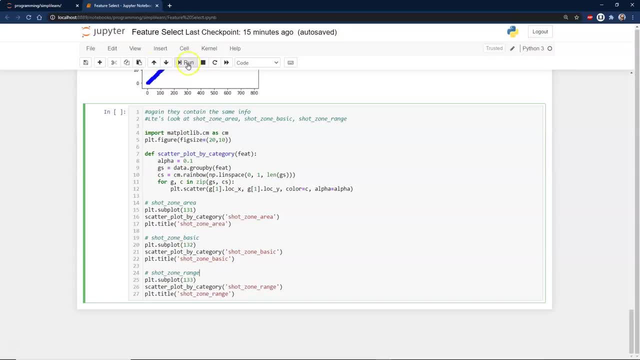 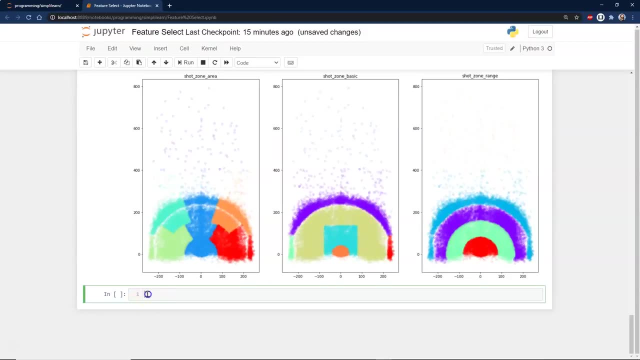 Again, it's a one by three set up and then it's just a place on each one, And so we look at this. we can see that these shots they map out the same. So it's very, again, redundant information that should be intuitive when we're looking at this in this color graphs. 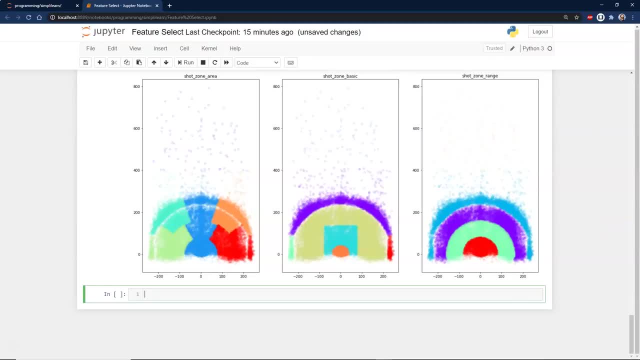 It kind of helps. you start looking at something you did- It's very intuitive, like this is- and you start to realize that some of this stuff You'll be looking for in data You might not understand. and you'll see these circular patterns where they match, or they mostly match, and you start to realize when you're looking at these that they're repetitive data. 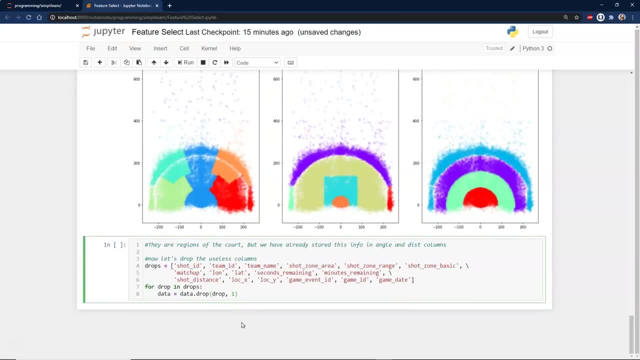 Then you want to explore them more closely, depending on what domain you're working in. So we look at these and we look at them and they look just like the regions of the court, but we already have stored this information and angle and distance columns. 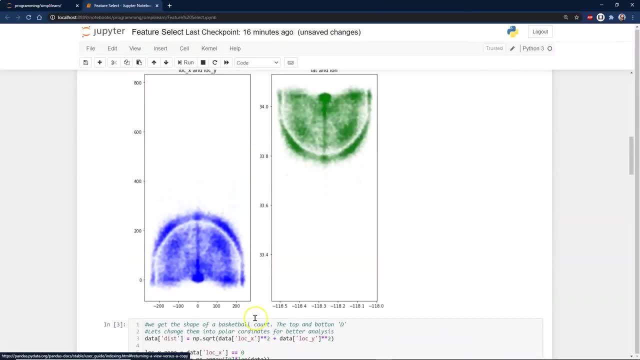 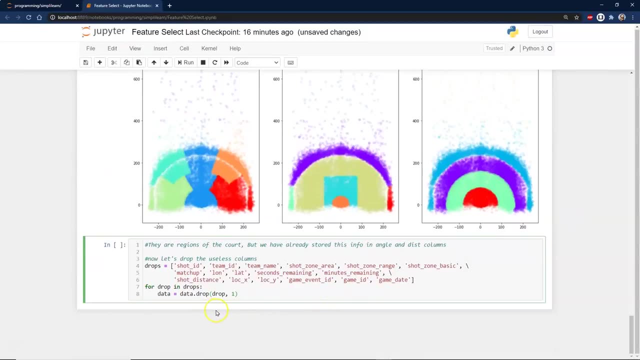 So we've seen this image before we go back up here and here's our. the similar image And repeating that image is down here, And so let's go ahead and drop some of this in this stuff. So now let's drop all the useless columns and we can drop the shot ID, team ID, team name. shot zone area. shot zone range, shot zone basic. the match up, the longitude and latitude. 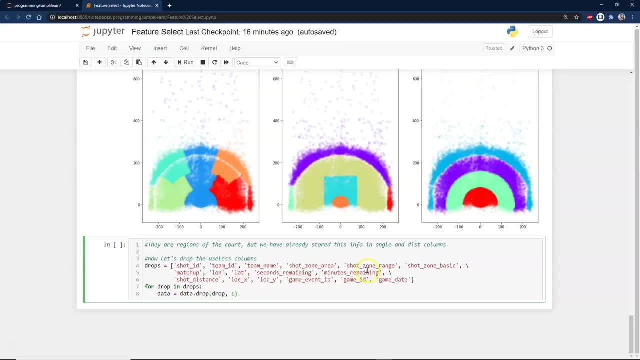 We're putting that into distance- seconds remaining, minutes remaining- because we combine that into one column: shot distance. because we have just distance on their location, X Location. Why the game event ID, game ID, all this stuff is just being dropped on here and we'll just go ahead and loop through our drops. 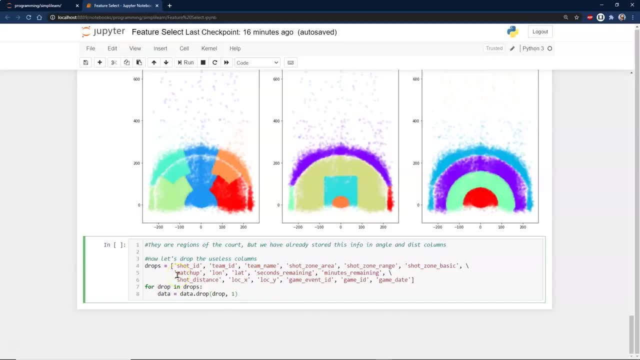 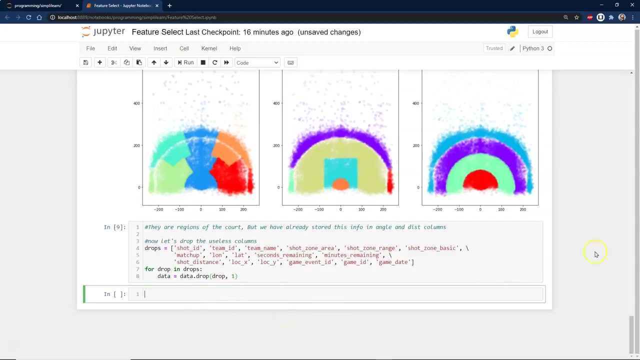 And this is a nice way of doing this because, as you're playing with this, this kind of data- putting your list into one setup- helps, because then you're just running it through an iteration and you can come back and change it. You might be playing with different models and do this with models. 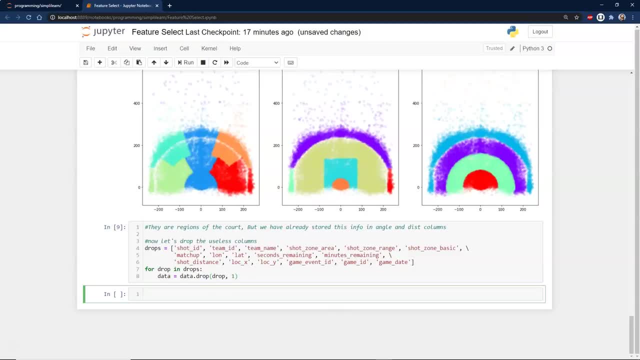 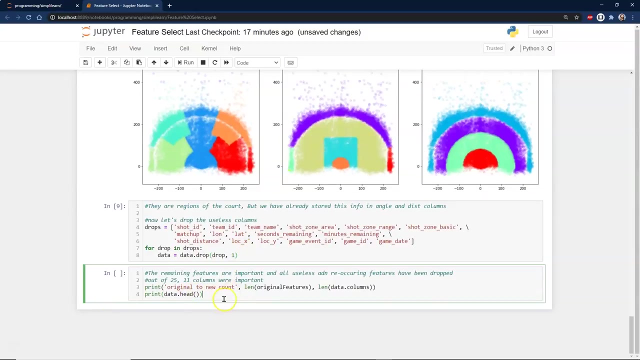 You might be looking at all kinds of different things that you can drop and add in as you test these These out and again. we're working in the filter method, So this is a lot of human interaction with the data, and it takes a lot of critical thinking to look at this stuff and say what matches and what doesn't. 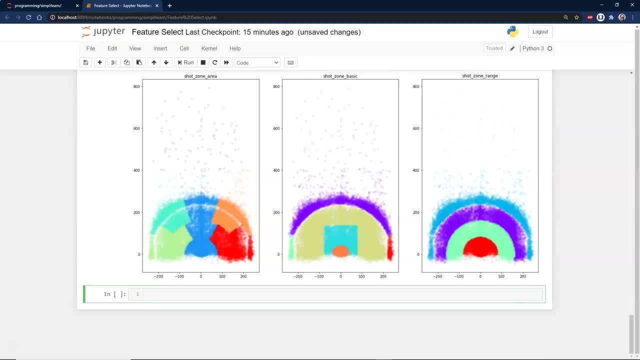 That should be intuitive. When we're looking at this in this color graphs, it kind of helps and you start looking at something you it's very intuitive- like this is, and you start to realize that some of this stuff you'll be looking for in data you might not understand. 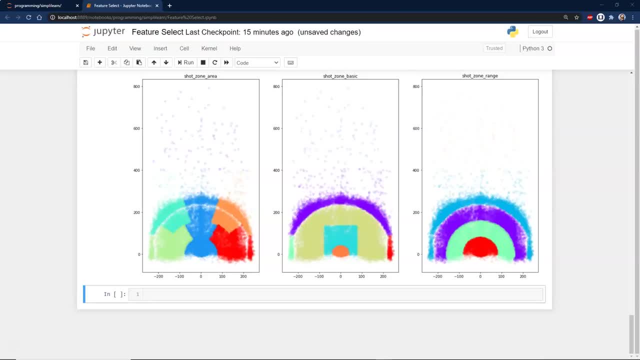 And you'll see these circular patterns where they match, or they mostly match, and you start to realize when you're looking at these that they're repetitive data and then you want to explore them more closely, depending on what domain you're working in. So we look at these and we look at them and they look just like the regions of the court. 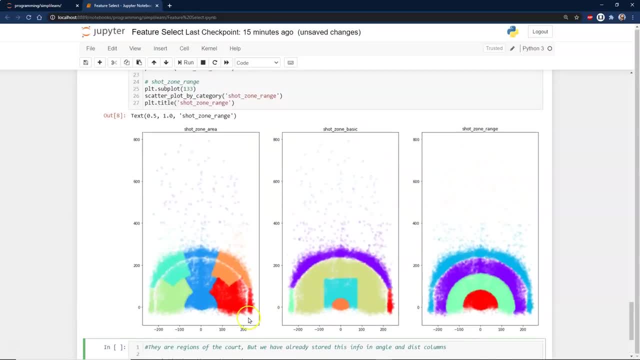 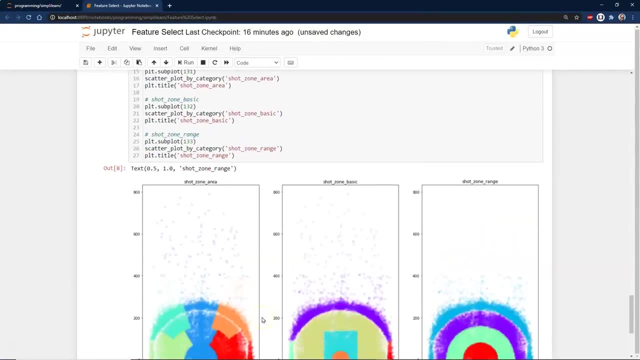 but we already have stored this information in angle and distance columns, So we've seen this image before. Let me go back up here and here's the similar image And repeating that image is down here, and so let's go ahead and drop some of this stuff. 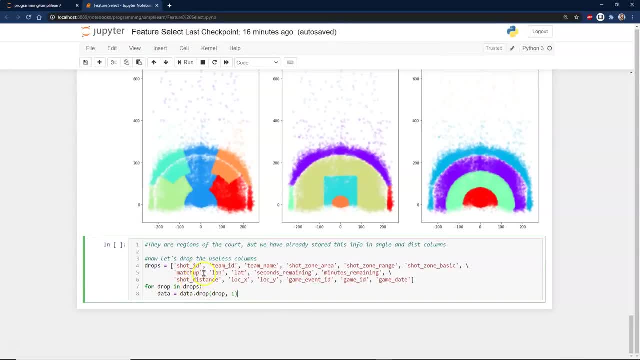 So now let's drop all the useless columns And we can drop the shot ID team ID team name. shot zone area. shot zone range. shot zone basic, the matchup, the longitude and latitude, because we're putting that into distance. 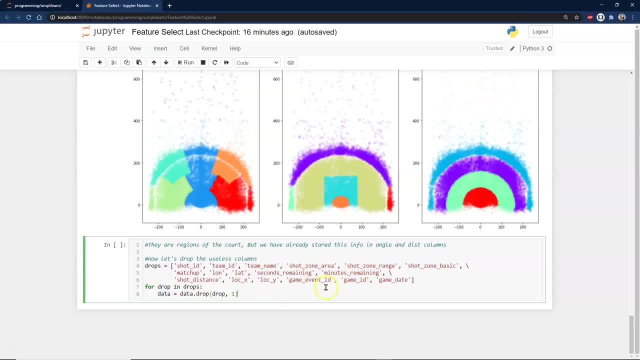 seconds remaining, minutes remaining, Because we combine that into one column Shot distance, because we have just distance on there. Location X, location Y, the game event ID, game ID, All of this stuff is just being dropped on here And we'll just go ahead and loop through our drops. 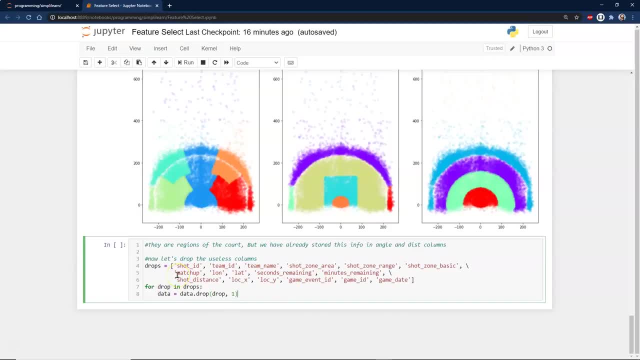 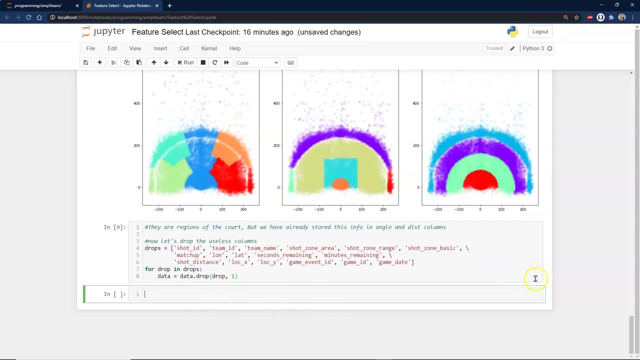 And this is a nice way of doing this because, as you're playing with this, this kind of data- putting your list into one setup- helps, because then you're just running it through an iteration and you can come back and change it. You might be playing with different models and do this with models. 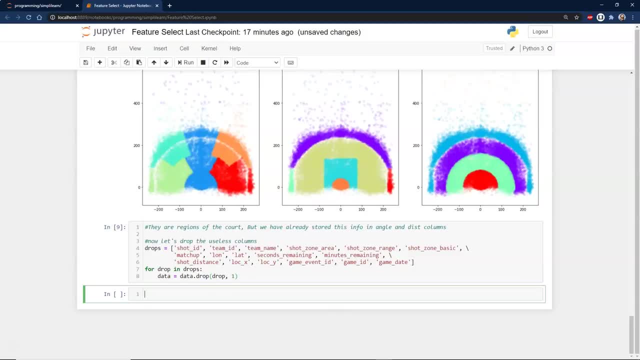 You might be looking at all kinds of different things that you can drop and add in as you test these out. And again, we're working in the filter method. So this is a lot of human interaction with the data And it takes a lot of critical thinking to look at this stuff and say what matches and what doesn't. 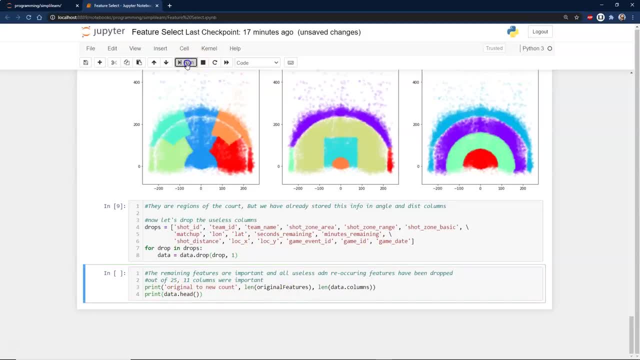 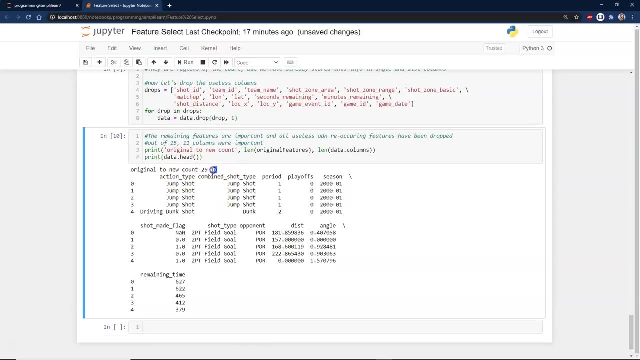 And so when we look at the remaining features- let me go ahead and just run this, The original, to the new count. we had 25 features, Now we have 11 features. You can see that right there. Just circle that. There's our 25, and there's old, new.